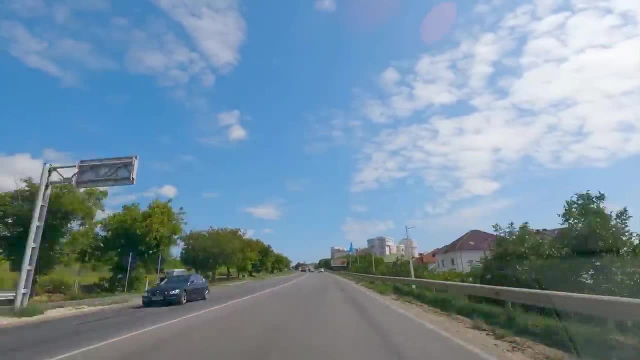 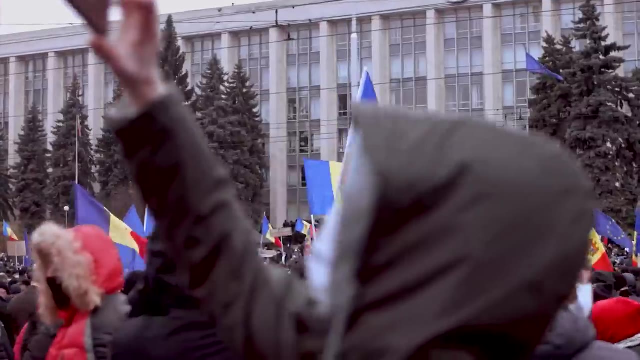 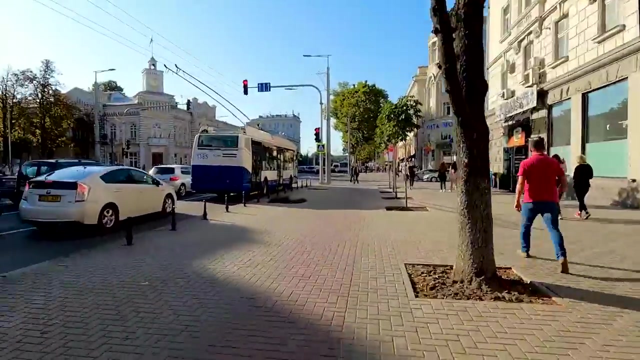 second lowest GDP per capita and hardly any infrastructure Existing outside the capital, Chisinau, which is often ranked as Europe's ugliest, most boring. capital Throw in a corrupt government and high levels of organized crime, and Moldovans are the least happy people on earth. No, like literally when pollsters ask. 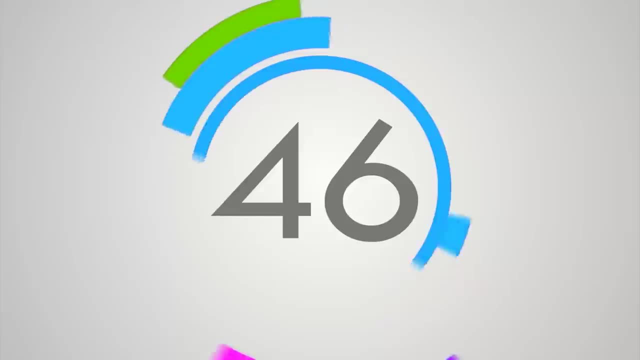 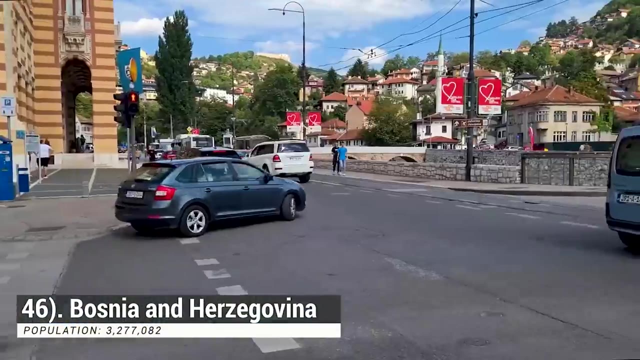 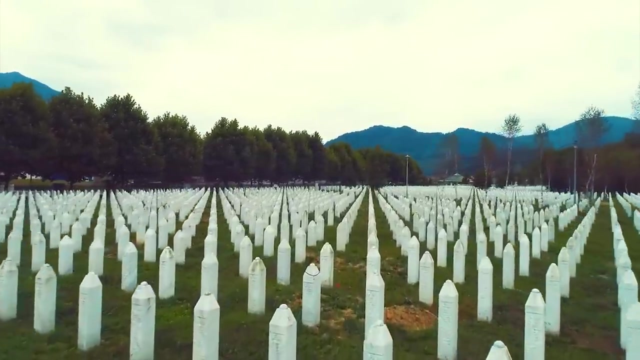 are you happy? More than half of Moldovans say no. Number 46,: Bosnia and Herzegovina. Bosnia and Herzegovina has been through a lot After the breakup of Yugoslavia in 1991, 8,000 Bosnians were murdered and 2 million displaced during the ensuing Yugoslav and. Bosnian wars And many ripples are still felt today, with the worst pollution in Europe, hundreds of completely destroyed buildings and extreme poverty and PTSD among its residents. Now those were the 5 worst countries in Europe, and before we get to the other 45,. 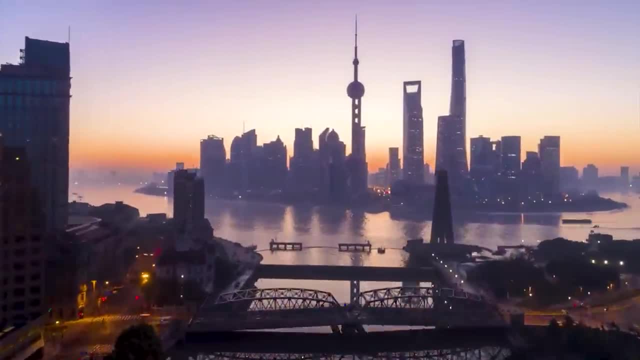 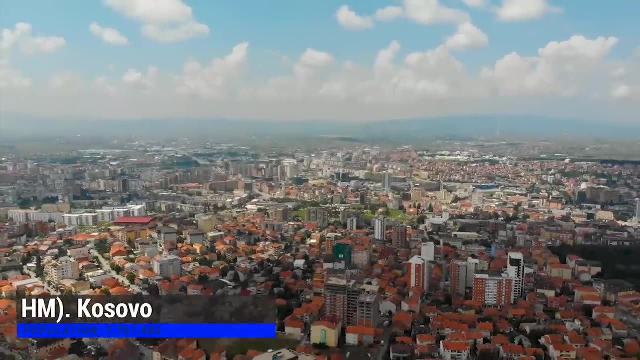 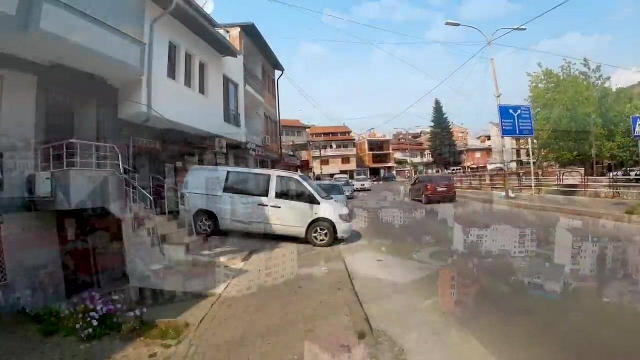 leave a like and subscribe. If we hit 10,000 likes, I'll rank every country in Asia too, And I also wanted to give an honorable mention to Kosovo, which Serbia claims It's the second poorest nation in Europe, with a terrible economy and the highest unemployment rate, at 20.6%. 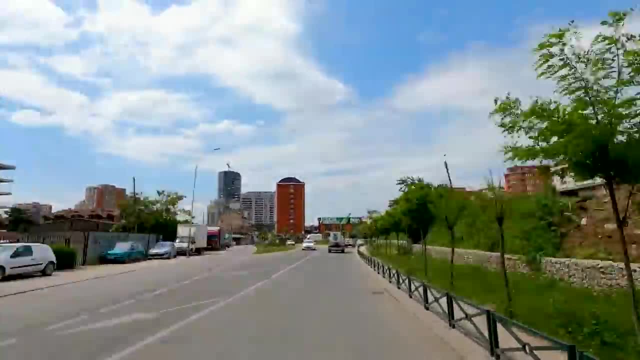 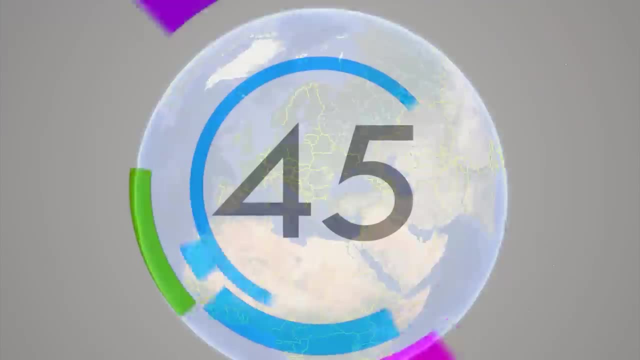 But since Kosovars receive a lot of money from displaced family members living in wealthier nations, the quality of life isn't terrible and average life expectancy is nearly 80.. Number 45, Azerbaijan. Wait a second. isn't Azerbaijan in? 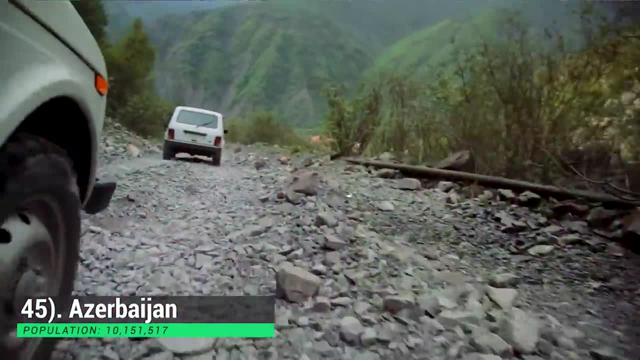 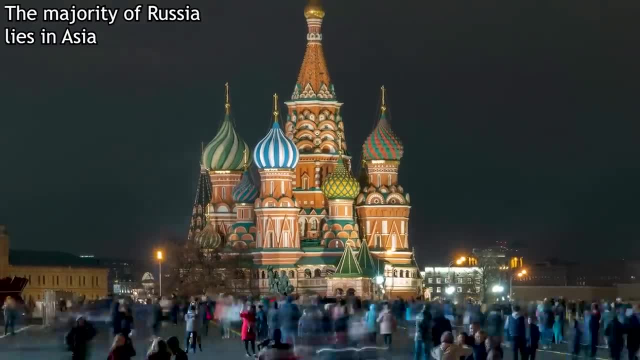 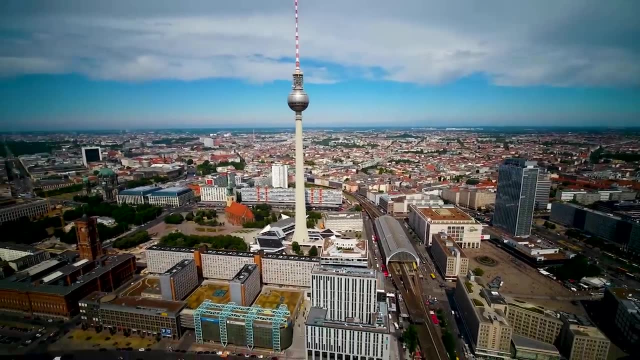 only 43 nations lie entirely within Europe's borders, But most organizations count 50 European nations and scientifically speaking, Europe isn't even a real continent, but rather a part of Eurasia. so its boundaries are mostly just political. And speaking of political, 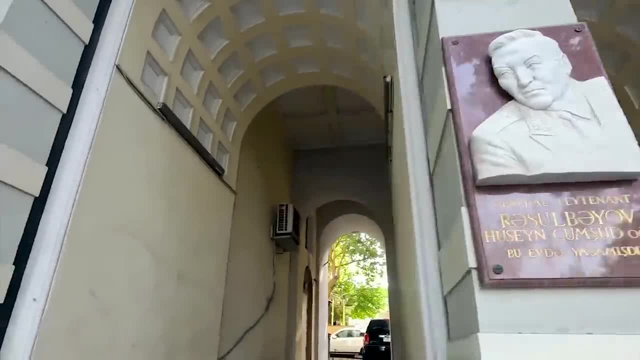 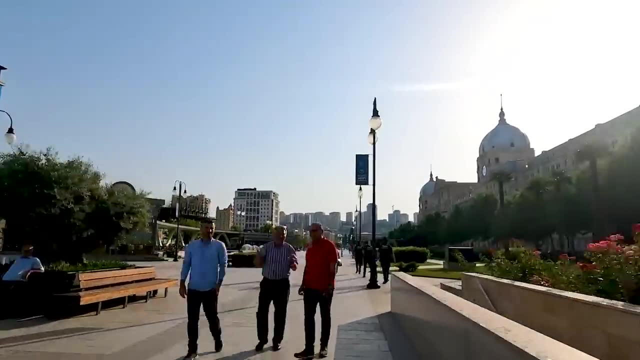 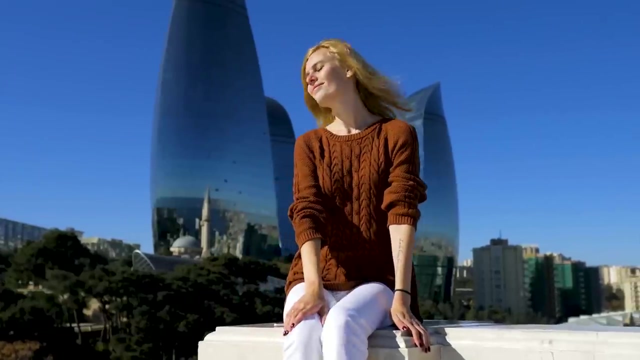 although Azerbaijan has the most secular government amongst majority Muslim nations, it's still egregiously authoritarian. Elections are not free or fair, political opponents are often imprisoned and the president and his father have had complete control of the country for 30 years. But due to its vast oil, 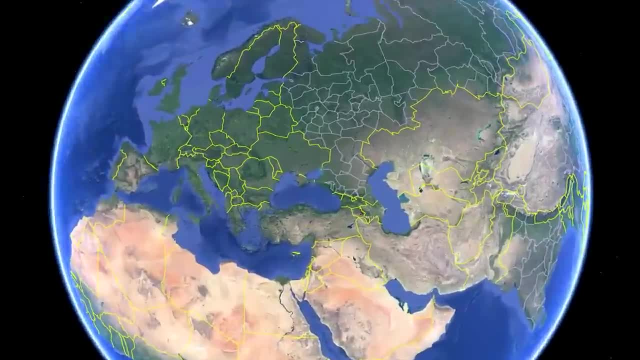 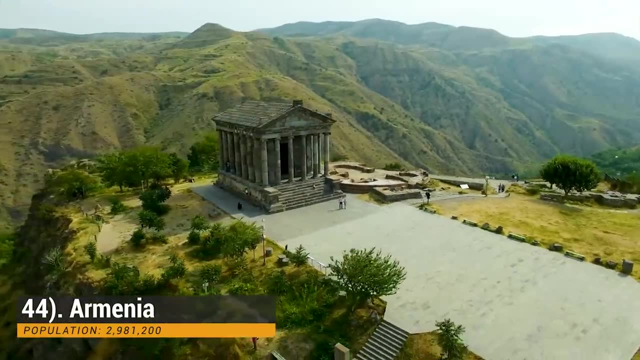 reserves. the economy is decent. Number 44, Armenia. Geographically speaking, all of Armenia lies in Asia. Geopolitically and culturally, however, it's very European and part of most European groups, such as the Council of Europe. But Europe or not, 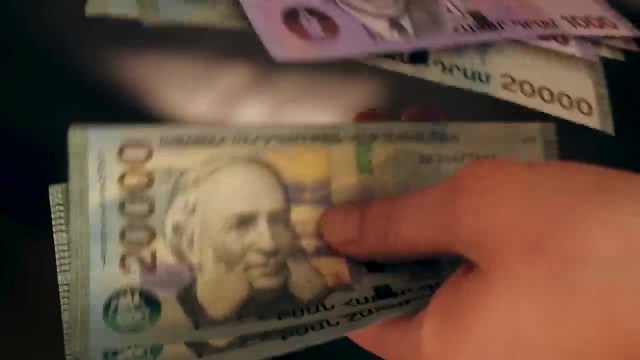 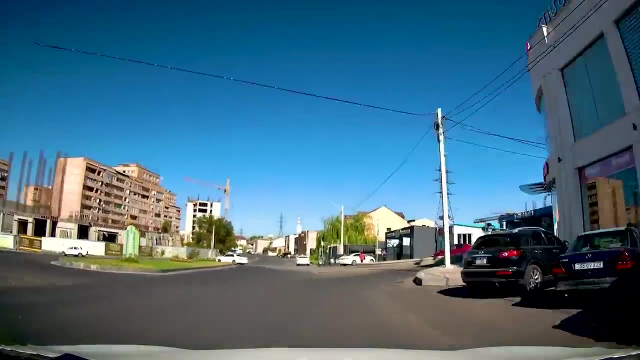 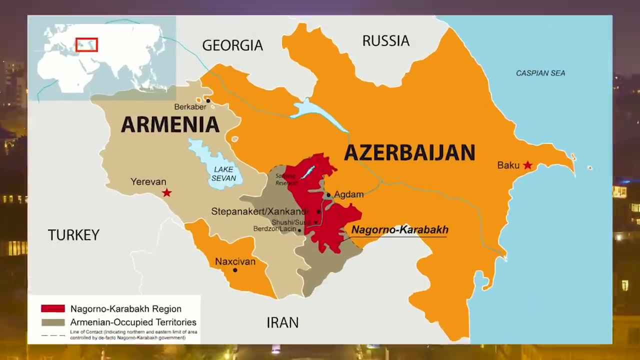 26.5% of Armenians live in poverty because, despite the political system being more democratic than Azerbaijan's, it's still incredibly corrupt, leading to little economic opportunity. This combined with the nation's near-constant conflict with Azerbaijan over the disputed Nagorno-Karabakh territory. 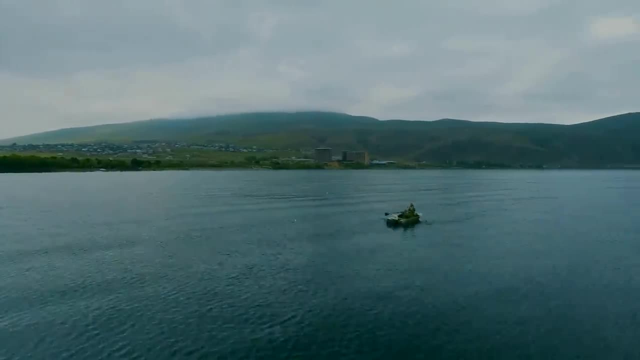 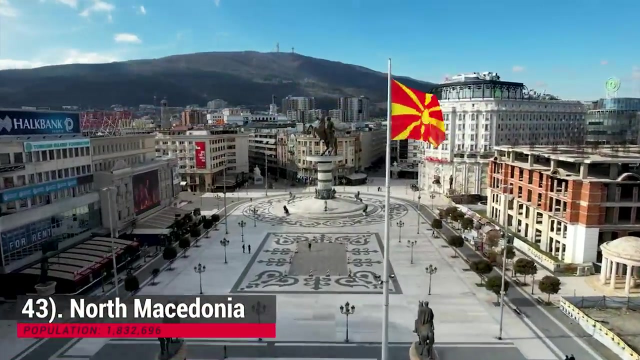 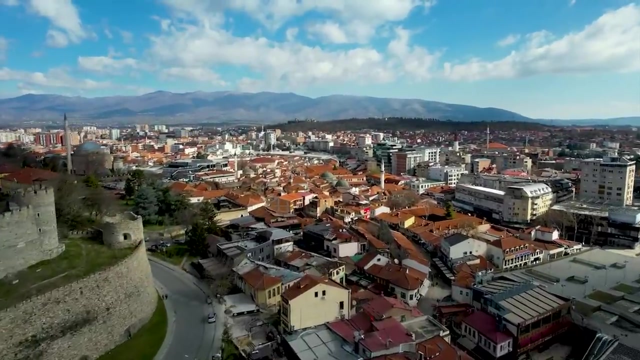 has resulted in the displacement of hundreds of thousands of Armenians. Number 43,: North Macedonia. After countless controversies with Greece regarding the name Macedonia and its former, excessively long name, former Yugoslavic Republic of Macedonia, the nation was officially renamed North Macedonia in 2019.. But, unlike the vast 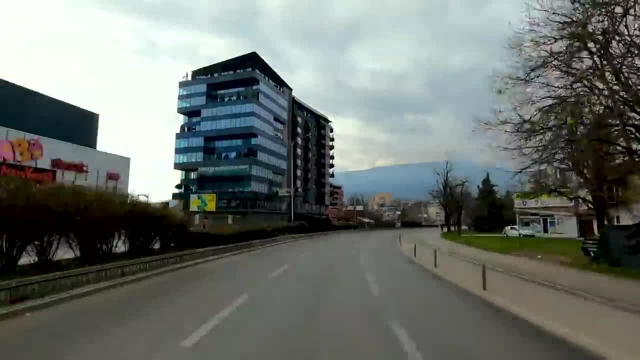 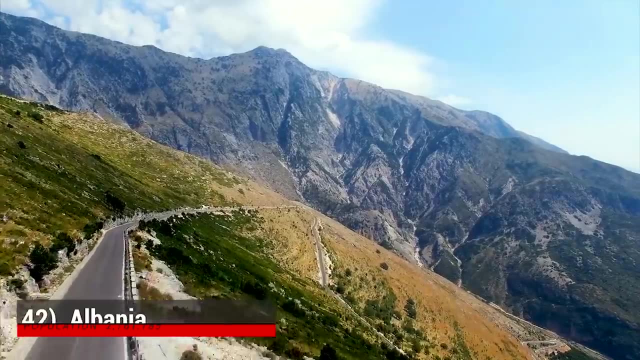 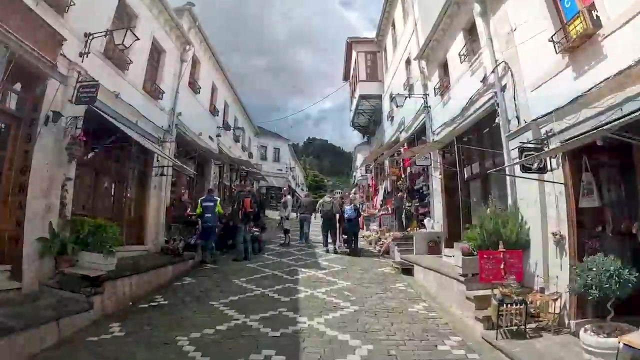 Macedonian Empire Alexander the Great once led. the only thing North Macedonia is leading the continent in is unemployment Number 42, Albania. While it's likely the most beautiful European nation that you know nothing about, Albania is not a great place to live, But considering their 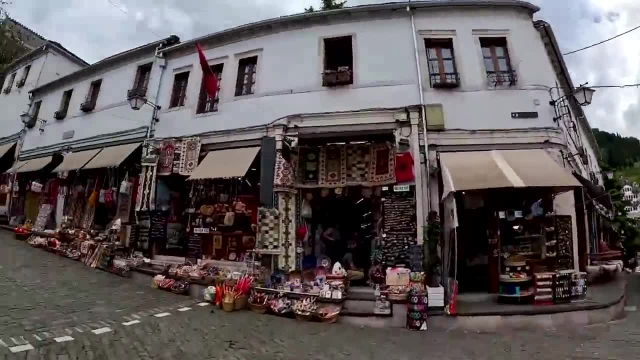 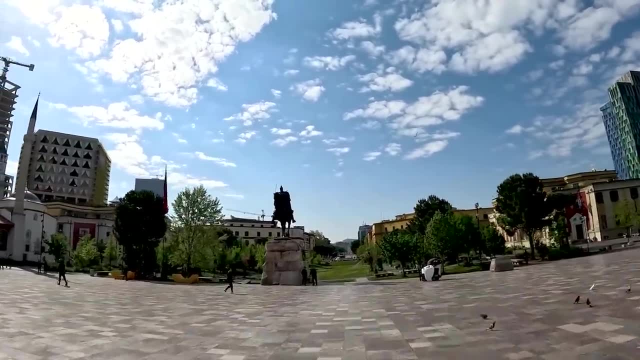 tragic history. it's a miracle Albania has recovered at all After being under one of the most impoverishing conditions in the world. Albania is now a great place to live, But for half a century, with the former lunatic dictator using the nation's money to build nearly 200,000 bunkers for an invasion that never came. the new democratically elected government in 1992 proceeded to lure two-thirds of the population into a government-backed pyramid scheme which obviously failed, bankrupting the majority of Albanians and resulting in the 1997 Civil War. 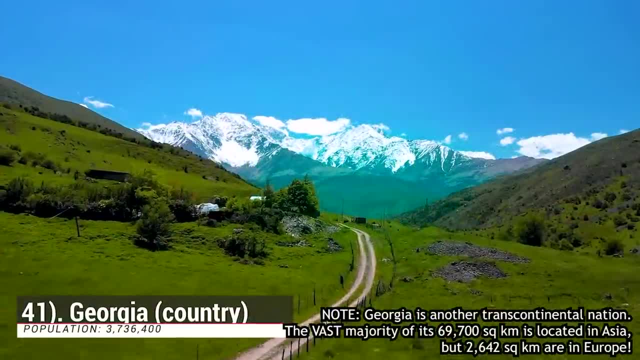 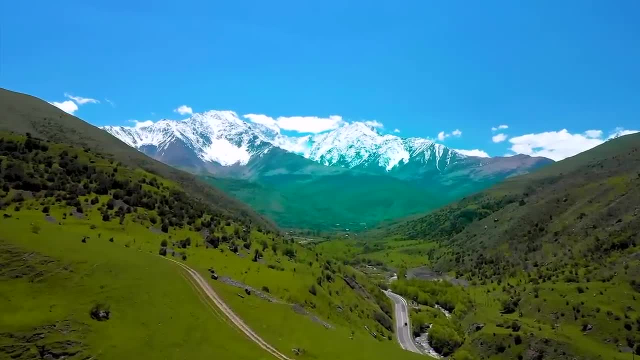 Number 41, Georgia. Georgia is Europe's most homophobic nation, with 84% of the population of residents saying same-sex relations between adults is always wrong, And this stubborn mentality opposing progress translates to all aspects of life. Average wages have remained low. 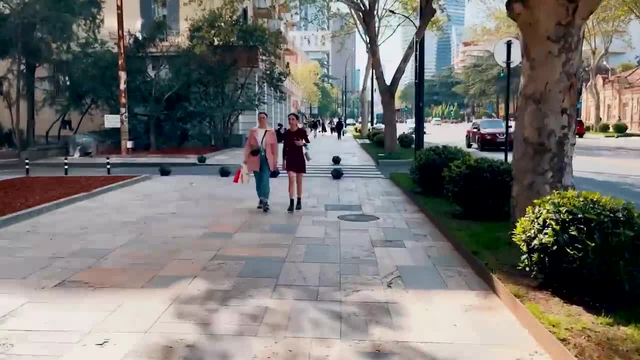 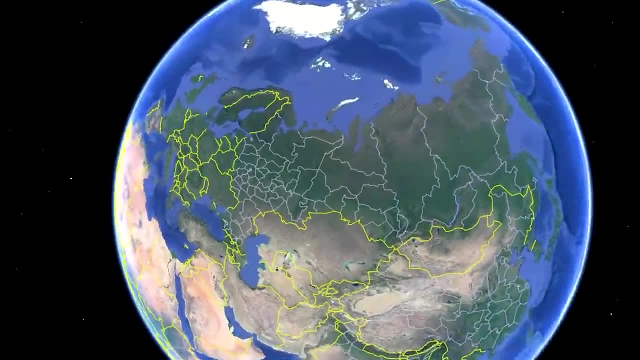 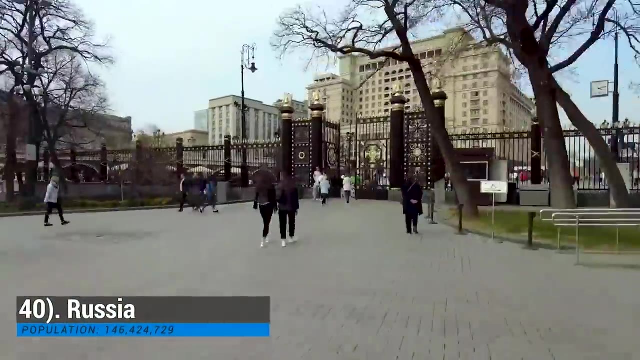 healthcare and education remains poor, and its cities are among the most polluted on earth, resulting in a life expectancy that's lower than Syria. Number 40, Russia. Let's just get this out of the way. Russia has extremely limited personal freedoms. There's no right to peaceful assembly and public 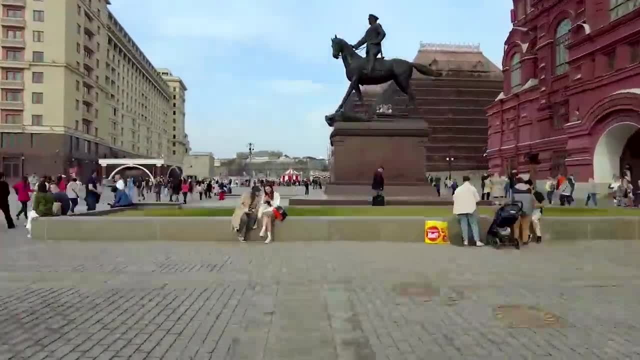 opposition to the rule of law. Russia has no right to peaceful assembly and public opposition to the rule of law. Russia has no right to peaceful assembly and public opposition to the rule of law. Russia has no right to to the war with Ukraine, or even calling it a war is considered a crime. But for all its issues. including being Europe's most corrupt and dangerous nation. it's cheap and the economy and infrastructure, especially in Moscow and St Petersburg, is very advanced, with the world's sixth-highest GDP at purchasing power parity. Number 39, Serbia. Belgrade, the former capital. 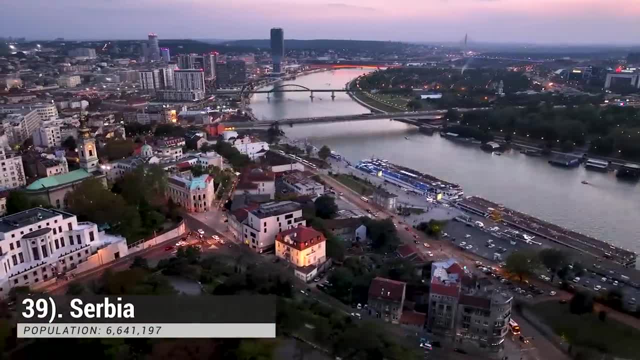 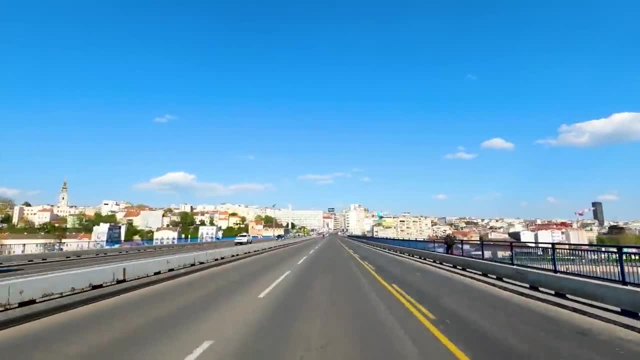 of communist Yugoslavia is now Serbia's capital and a party capital with the lonely planet, ranking at the number one position in the world's most corrupt and dangerous nation. But for all its issues, in this city of extremes with its beautiful historic center and flashy business-oriented, 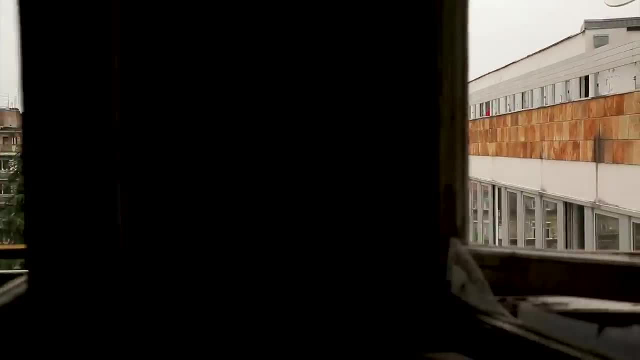 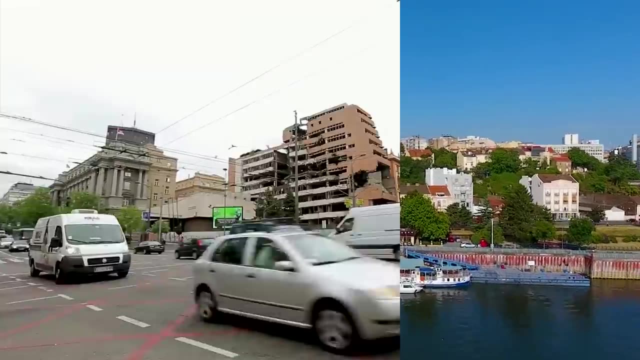 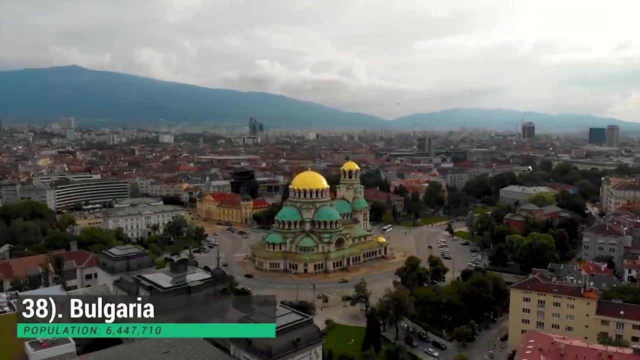 new Belgrade, sitting next to destitute districts without proper sewage, represents the nation at large. If you have money, it's great. If you don't, it's not. Most people don't. Number 38, Bulgaria. Bulgaria is one of the most fascinating countries. It's the only Slavic state. 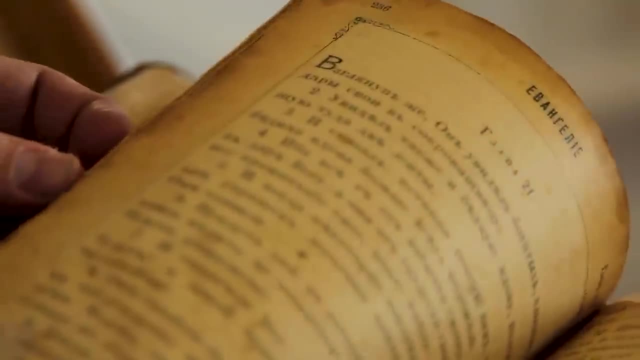 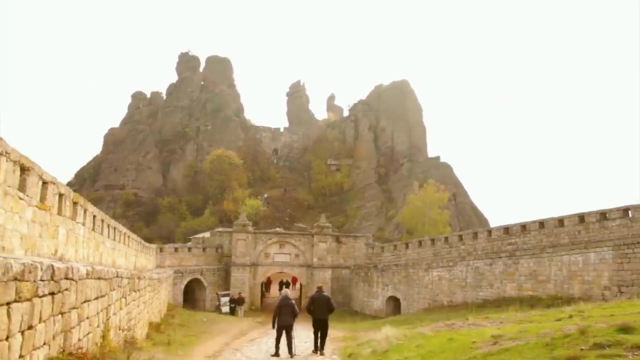 to never join Yugoslavia. The Cyrillic alphabet was invented here and it's home to the most archaeological sites in Europe other than Greece and Italy. But it's also full of contradiction. While its merit-based schools are remarkable, the majority of schools suck. While its 59-week 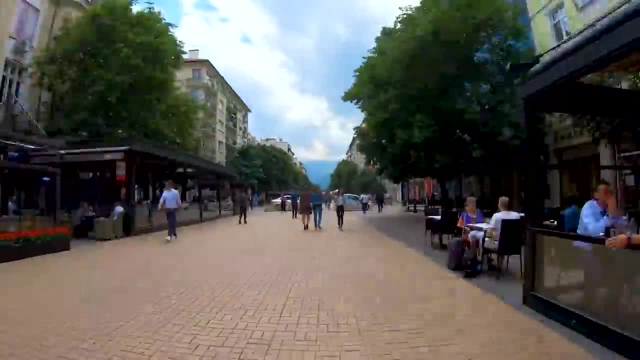 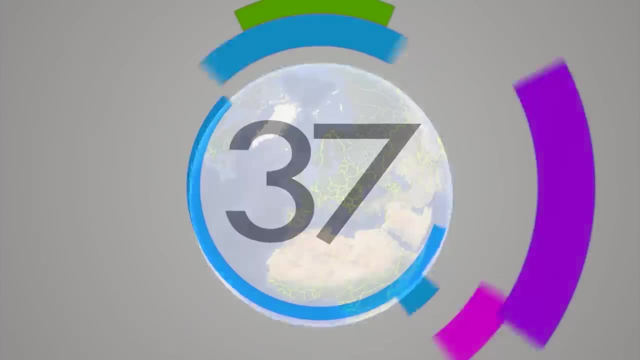 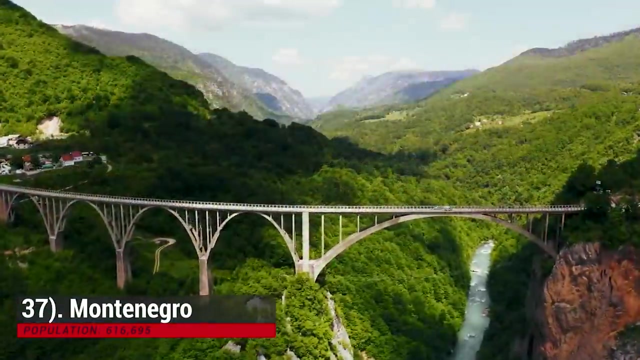 paid maternity leave is the highest in Europe, so is the mortality rate, And while the GDP per capita isn't terrible, 23% of the nation still lives in poverty. Number 37,: Montenegro. Before five seconds ago, most of you had never heard of Montenegro, And even now some of you are probably. 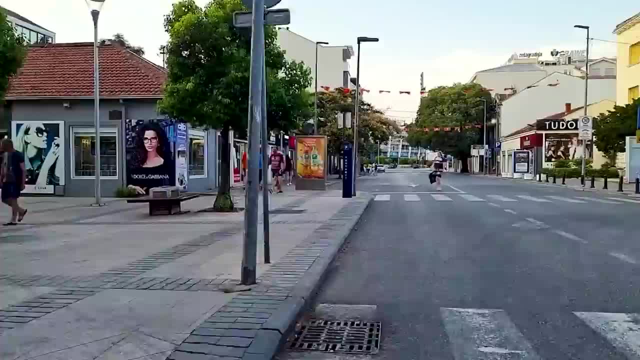 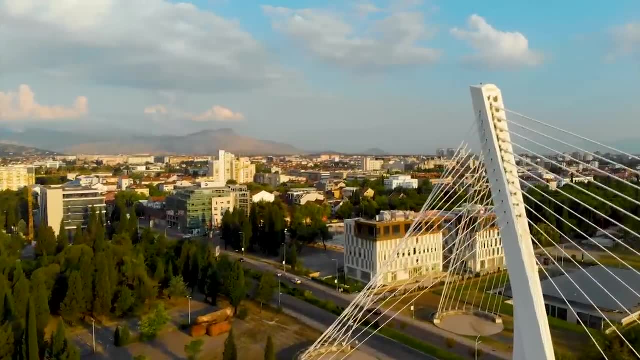 questioning: wait, does Montenegro exist? But although this unknown nation of 600,000 really tall people is the least corrupt in the Balkans, which is a big reason why it's the non-EU member closest to joining, it's also tiny, with low wages and taxes resulting in severely underfunded. 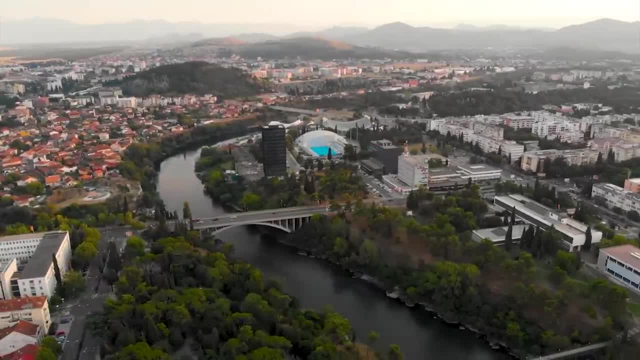 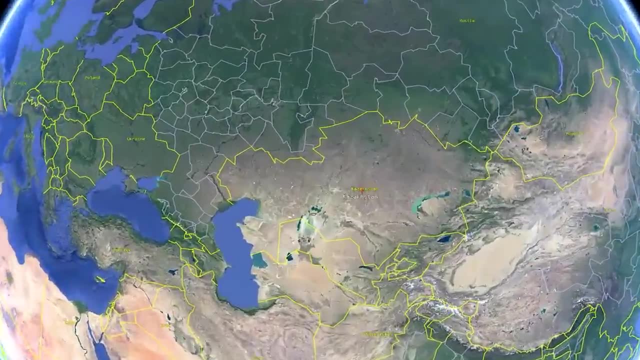 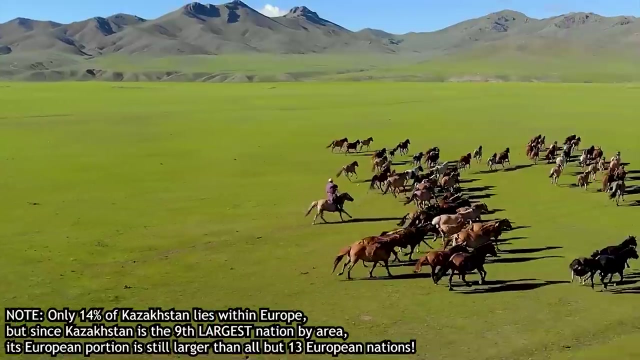 social programs. But hey, at least Montenegro owns the domain me- which actually pays the nation $350 million a year. Number 36, Kazakhstan. Apart from being almost nothing in Borat about glorious nation of Kazakhstan was true, But despite hardly exporting. any potassium. Kazakhstan is the greatest exporter of uranium, which, combined with the planet's 12th largest oil and gas reserves, have led to a stable, growing economy and highly developed cities and transportation. Number 35, Turkey. Turkey's most populous city, Istanbul, straddles. 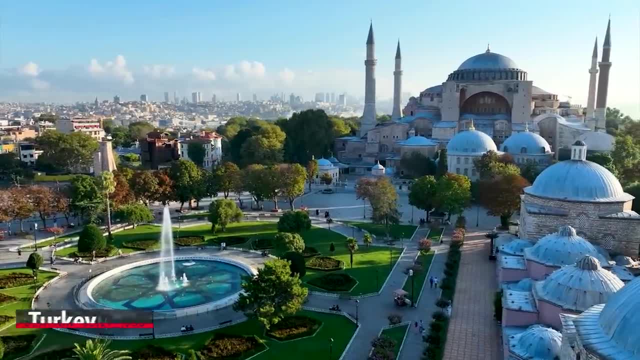 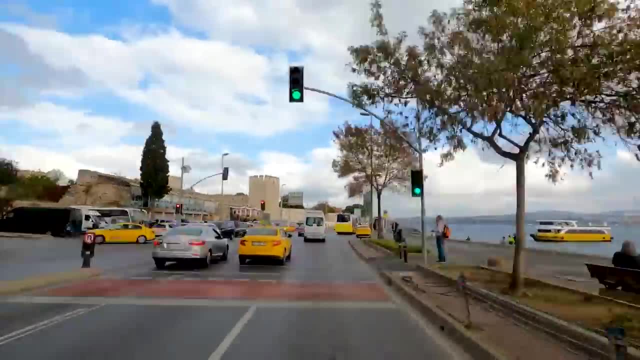 the border between Europe and Asia and has been one of the most important cultural centers for the nation for millennia. But while it and the European portion of Turkey is wealthy, accounting for 30% of the nation's GDP, despite covering just 3% of its land mass, most of Asian. 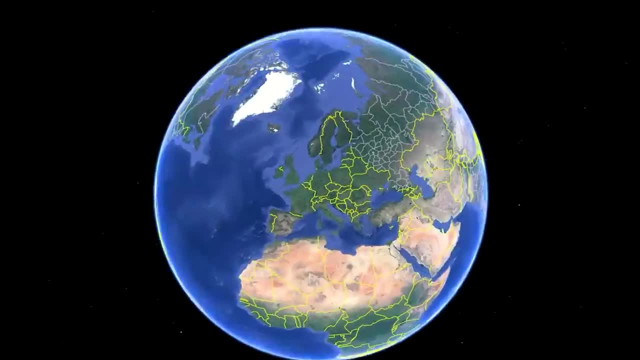 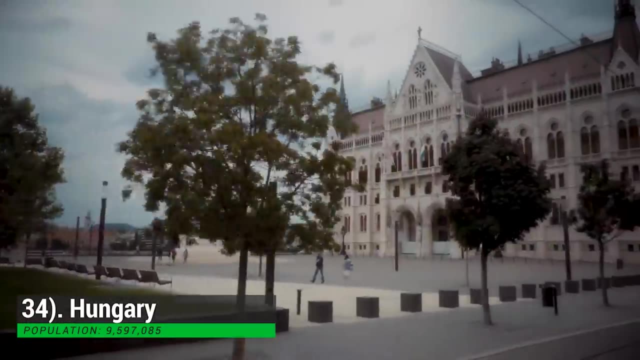 Turkey is extremely impoverished. Number 34, Hungary. Hungary receives one of the largest amounts of EU development funds, But since its government is by far the most corrupt in the EU, most of it is funneled to the prime minister's family and friends, rather than used to improve. 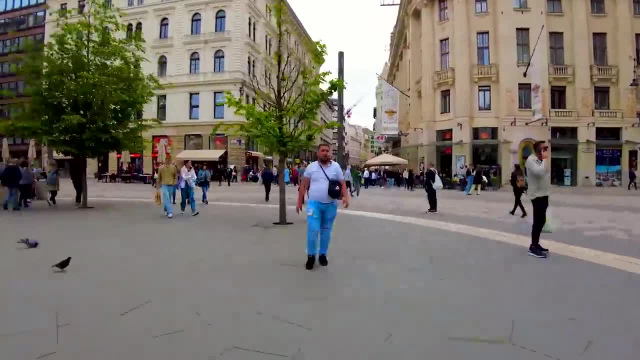 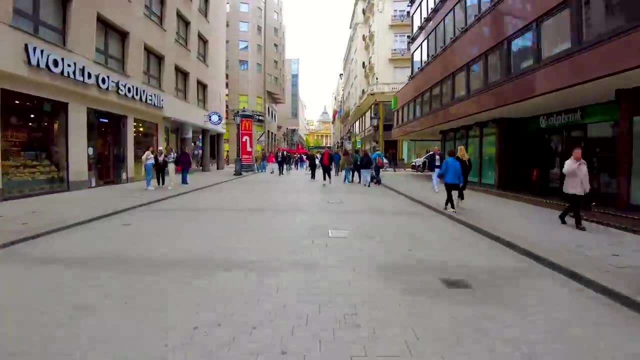 the nation's infrastructure or economy. Add on the world's health and security and the country's highest value-added tax at 27%, and the result is the worst inflation in Europe, with the nation's currency being devalued by 20% each year. No wonder Hungary has the most porn stars per capita. 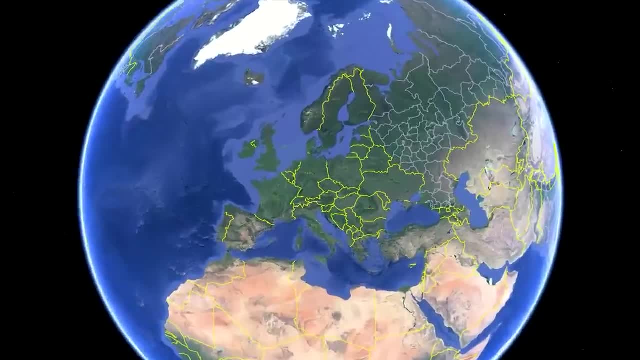 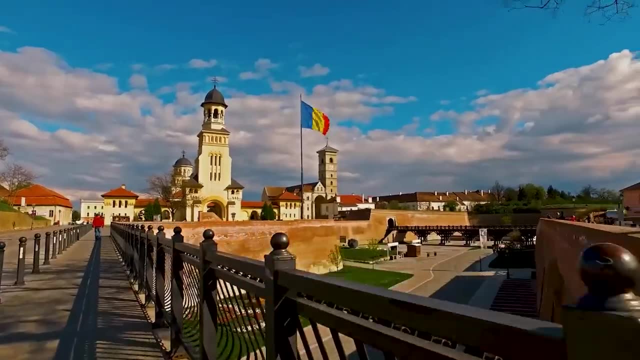 Only fans really do be saving lives. Number 33, Romania. While Hungary is the prime example of a nation's quality of life suffering due to corrupt governance, Romania is the opposite, being the poster child for how quickly a nation can turn things around. One of the poorest countries with 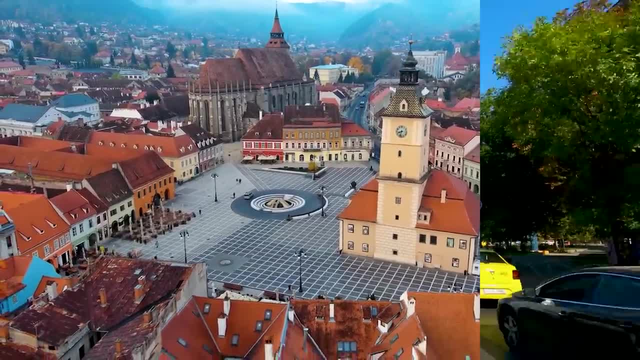 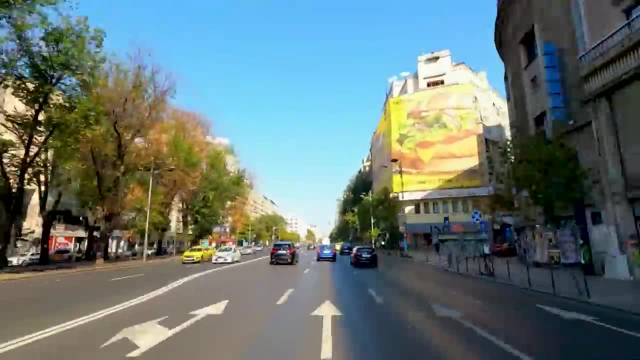 a rate of 42%. when admitted into the EU in 2006,, Romania has had Europe's fastest-growing economy ever since, with its GDP growing by 650% over the past 20 years, cutting the poverty rate to just 10%. 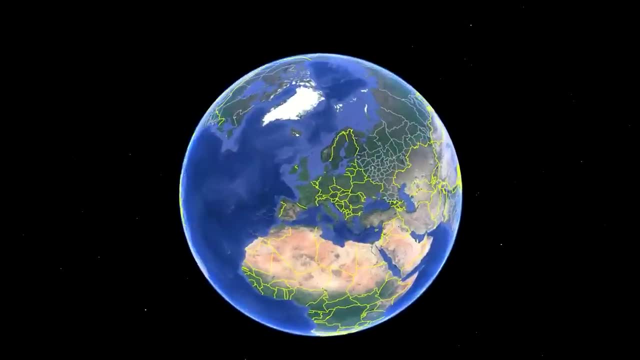 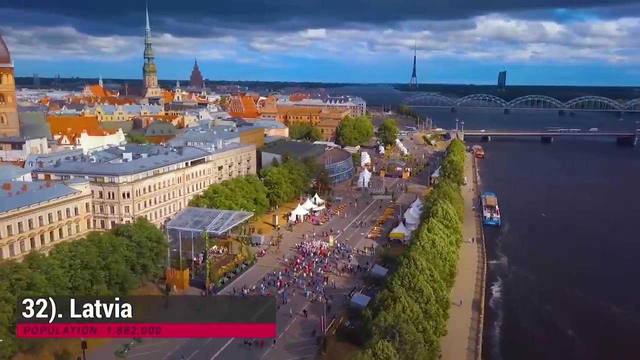 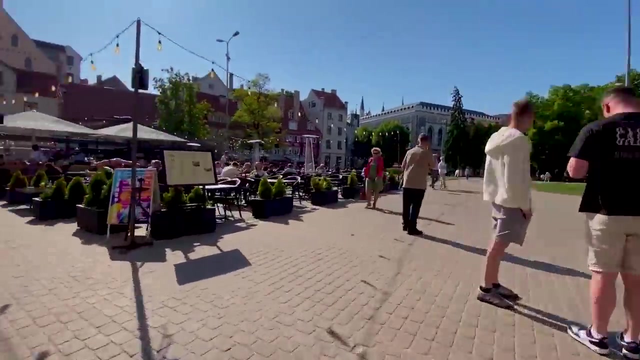 today. Oh, and Dracula lived here. Number 32, Latvia. Latvia houses more women than any other nation and has prospered greatly since the breakup of the USSR, But it's still the poorest and most inflation and roads in Europe. Number 31, Slovakia: No, not Slovenia. 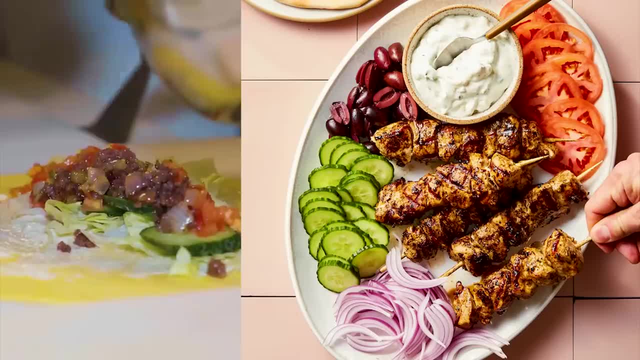 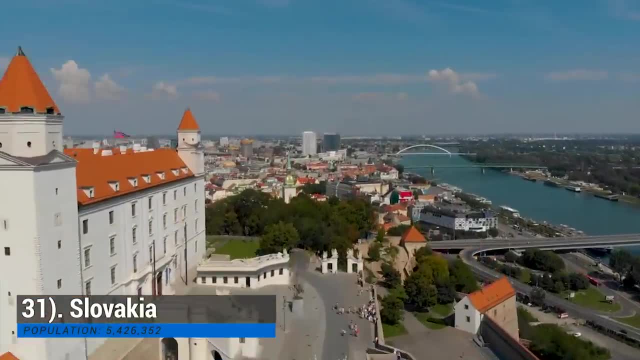 that's in the Balkans And not Slovaki. that's Greek And delicious. But while few of you can pronounce the former half of Czechoslovakia properly, and even fewer of you can locate it on a map, Slovakia has quietly been improving its quality of life, in large part due to producing 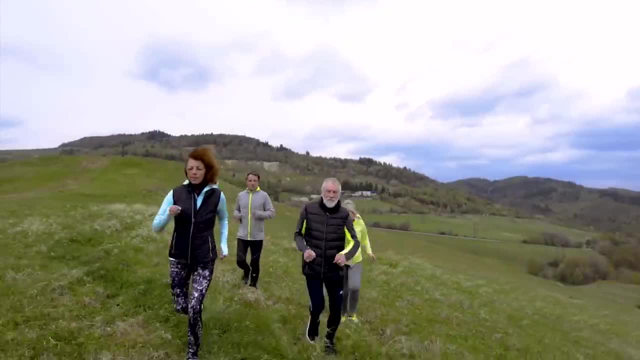 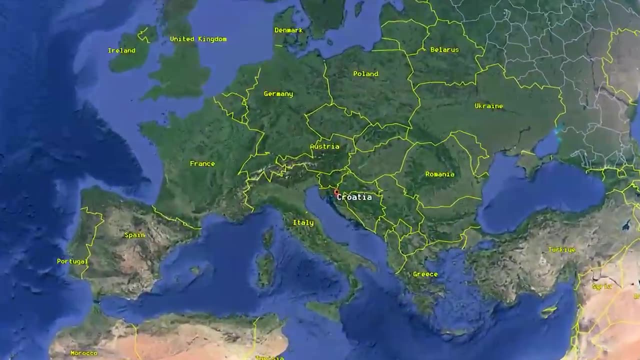 the most cars per capita. It's also incredibly safe. education and healthcare, is reliable and free, and its capital, Bratislava, even has a UFO Number 30, Croatia, Ever since joining the EU in 2013,. and people learning that much of Game of. 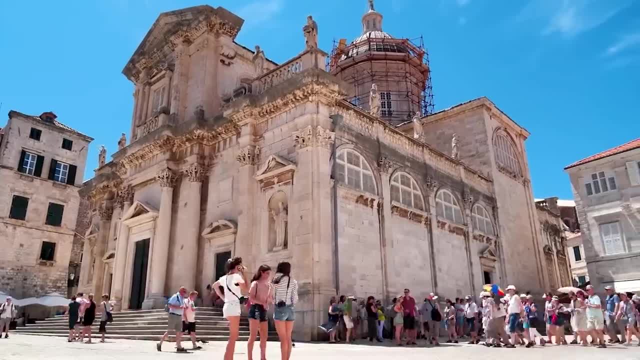 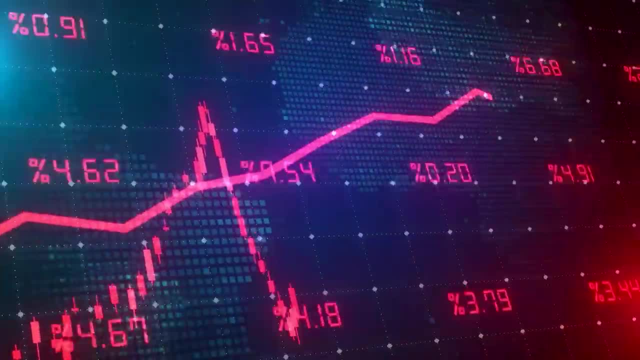 Thrones was filmed in Croatia. tourism numbers have skyrocketed, doubling from 2014 to 2019.. But this, in addition to the recent adoption of the Euro, has also led to prices rising, with the average cost of goods now being more expensive than Western Europe, despite salaries. 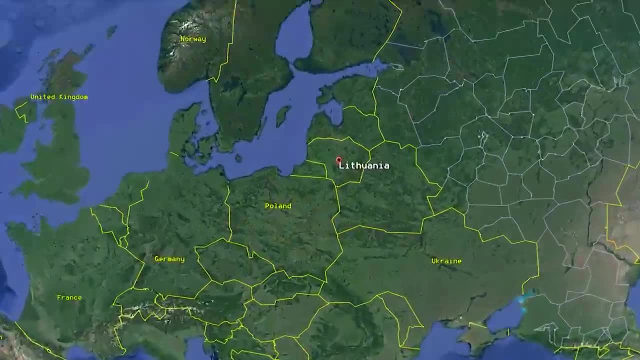 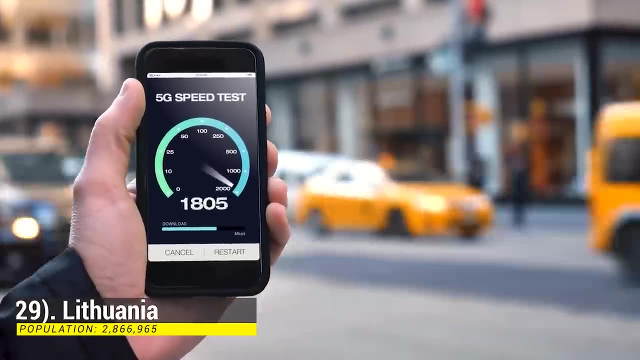 being much lower: Number 29,, Lithuania. If I lived in Lithuania, this video would've been uploaded on at least 8 minutes sooner, because it has the fastest internet on Earth, which is a testament to how far this small Baltic nation has come since they facilitated the breakup of the Soviet Union. 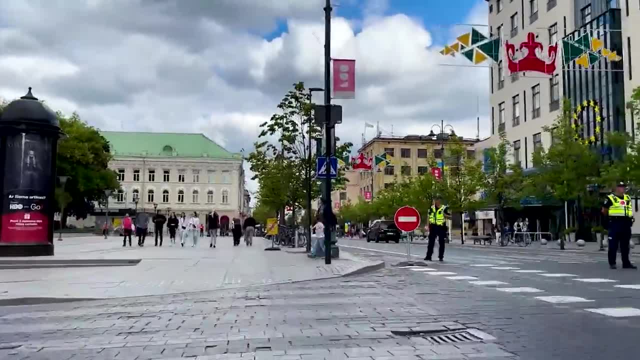 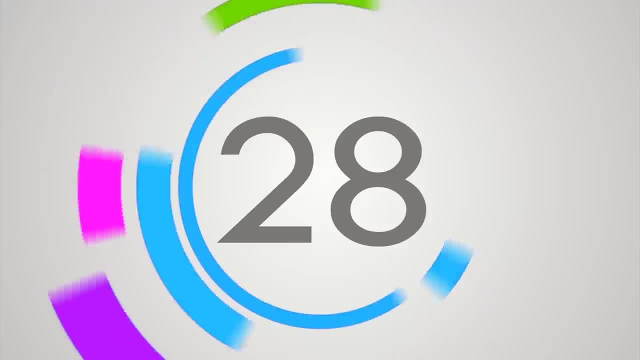 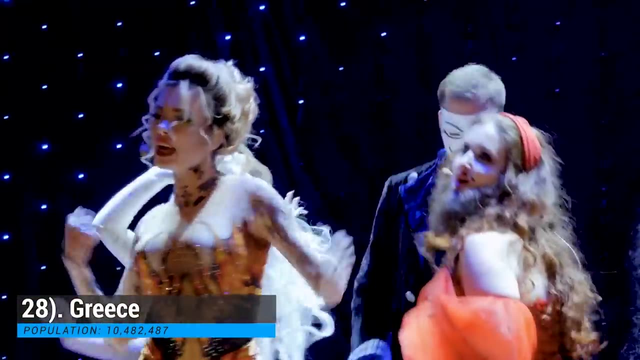 But although the economy has evolved greatly, many Lithuanians' worldviews have not, with most of the older generation being judgmental about anyone who expresses themselves. Number 28, Greece. Compared to the Balkans, Greece is wealthy. Compared to the EU, Greece is poor And compared. 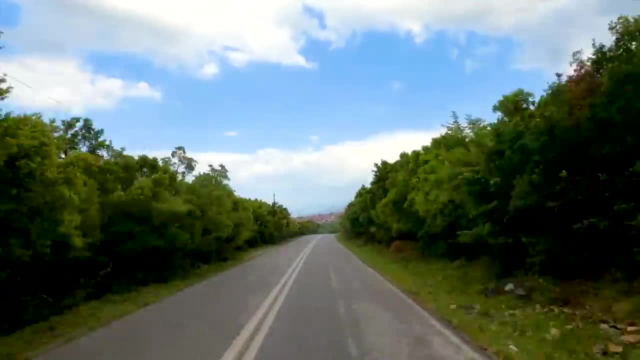 to musicals, Greece is the wealthiest country in the world. And, compared to musicals, Greece is the wealthiest country in the world. And, compared to musicals, Greece is the wealthiest country in the world. Its history, language and scenery are beautiful. the food is mouthwatering and healthy. 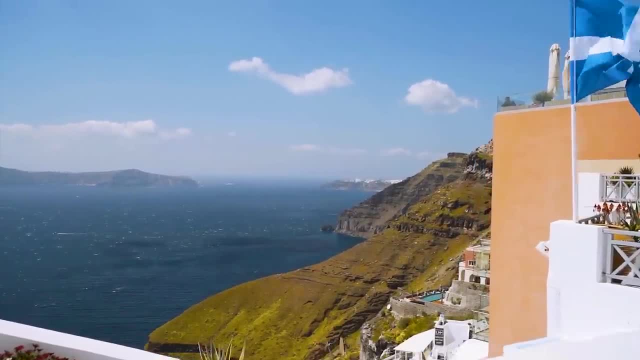 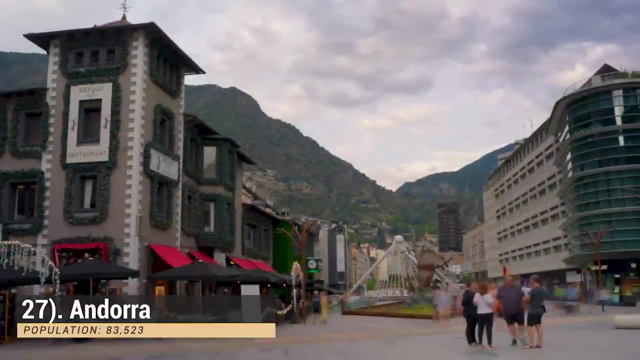 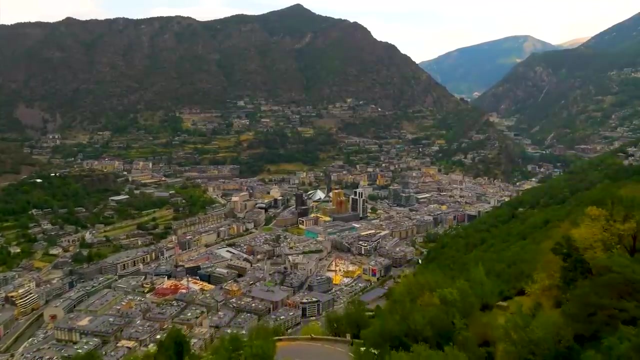 and its people are wonderfully warm and welcoming, despite their corrupt government and struggling economy. Number 27, Andorra. Skiing and duty-free shopping are the only reasons anyone ever thinks of this cheap 468 square kilometer nation. But you could also just go to Oregon for that. 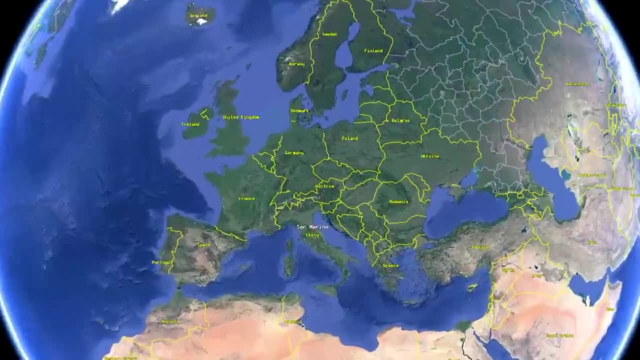 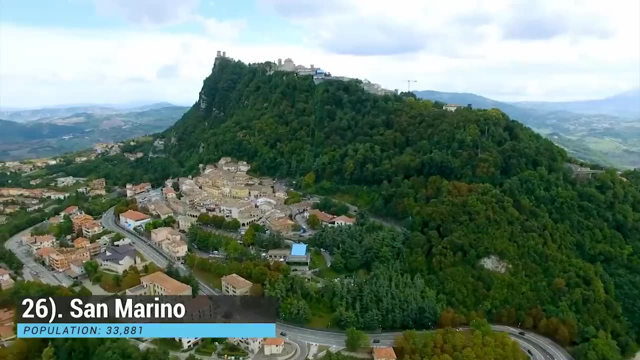 where there's better beer and legal weed. Number 26, San Marino. Andorra seems massive compared to this tiny 61 square kilometer microstate, which is located entirely within Italy and relies on it for 80% of its economy. But San Marino is also the oldest. 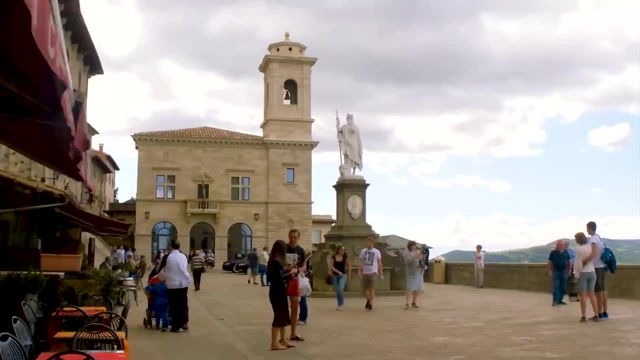 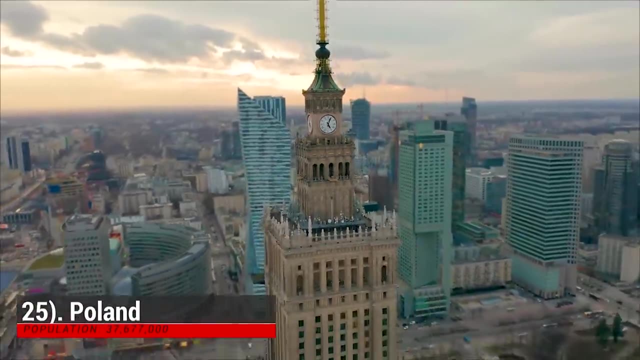 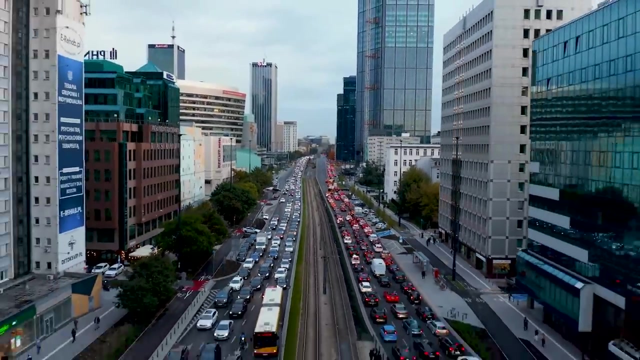 continuous country and exceptionally wealthy, with no national debt and the seventh highest GDP per capita, Number 25, Poland. Poland is the geographic center of Europe and also the center of this list because overall, it's pretty much the most average European nation. Well, a. 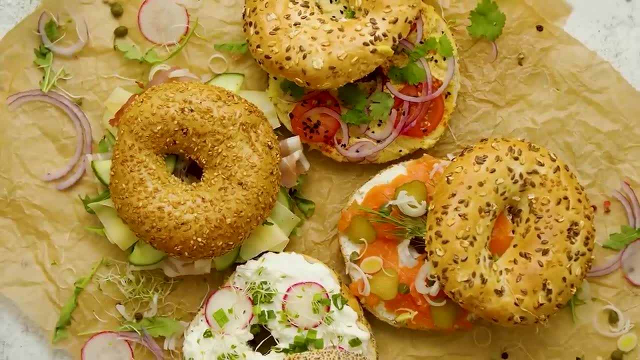 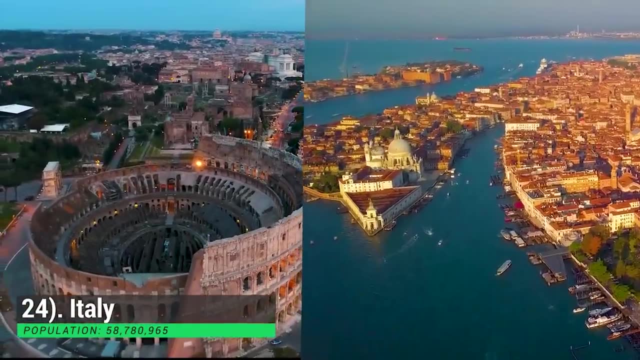 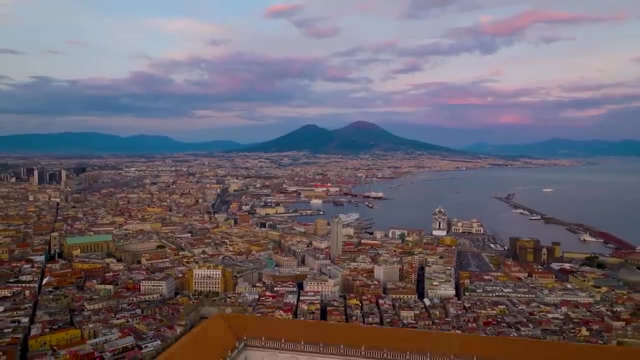 side from the fact that the godly delicatessen known as the bagel was invented here. Number 24, Italy. Italy is a tale of two nations. While the northern part is very rich and developed, with a quality of life similar to top ten countries, the south is really struggling. 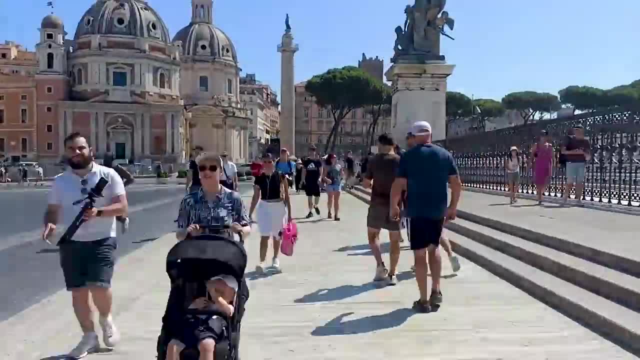 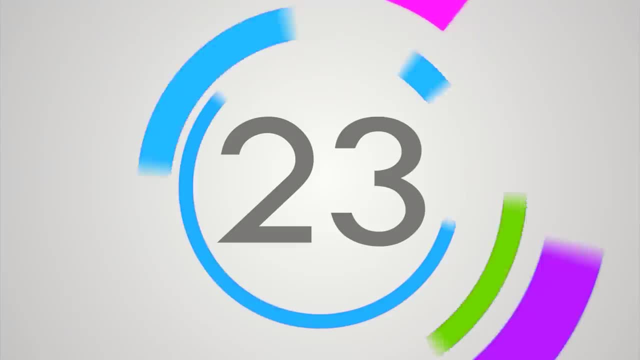 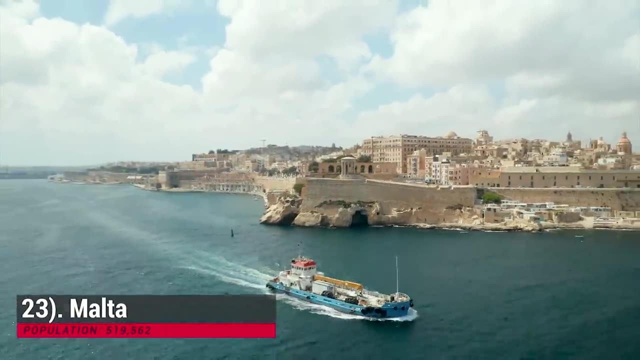 with less than half the north's GDP per capita and more than triple its poverty rate. Not to mention, it's got a real trash problem with Rome being named Europe's filthiest city, Number 23,. Malta, After having been colonized by 10 different empires over the last 2700 years. Malta, finally, 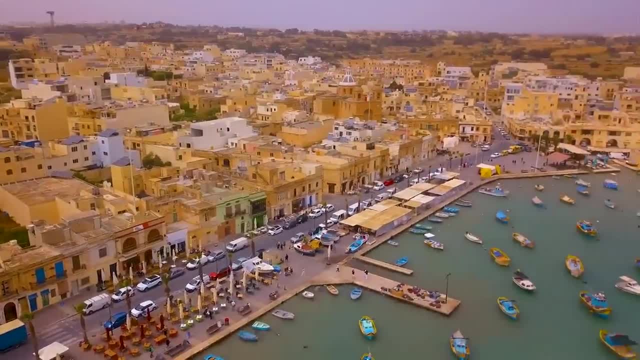 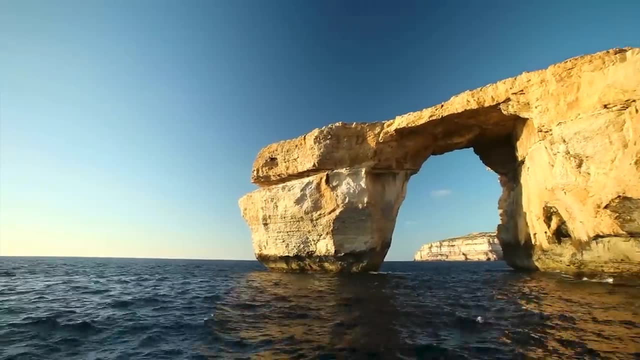 gained independence in 1964. And ever since, it's cemented itself as a tourist haven due to its year-round warm climate, awe-inspiring historic sites and world-class beaches, Not to mention. it's also become the iGaming capital of the world, which has resulted in high wages and Europe's 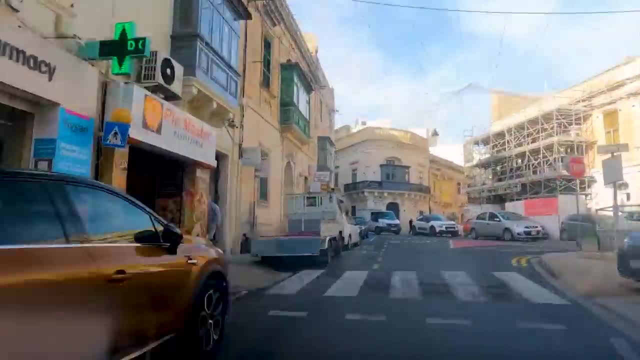 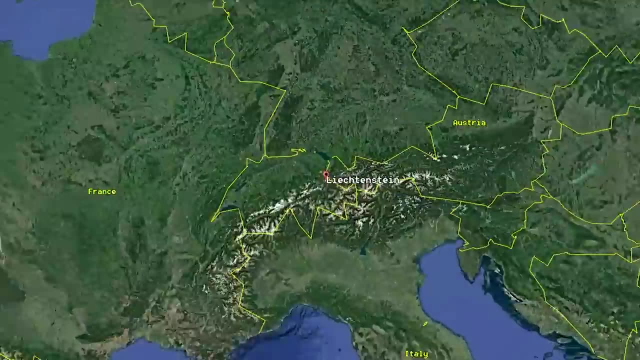 third-lowest unemployment rate. Oh, and, despite being Europe's most Catholic nation, Malta is also the most LGBT-friendly country in the world- Number 25,- Italy. Italy is also the most LGBT-friendly nation- Number 22, Liechtenstein. Liechtenstein is so small and irrelevant that even its neighbor 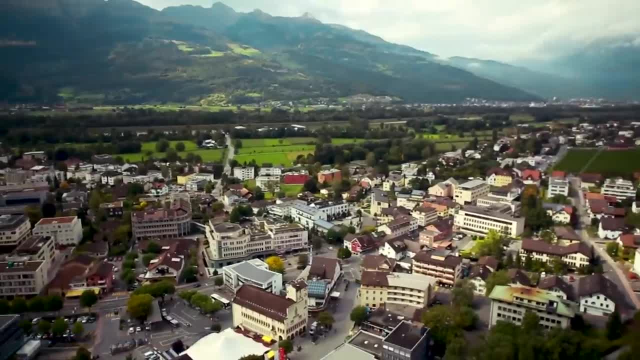 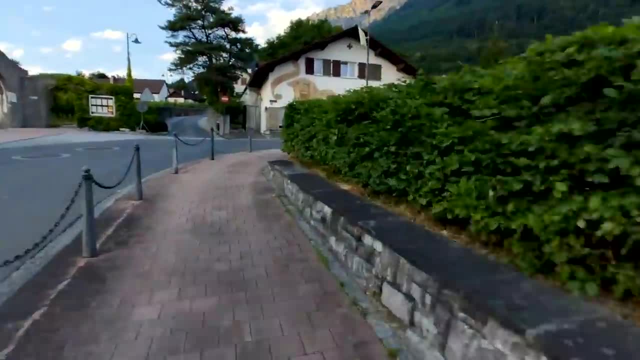 Switzerland often forgets it exists, having accidentally invaded the nation five times, And up until a decade ago you could actually rent the entire country for just 70 grand a night. But despite nothing noteworthy ever having happened here, Liechtenstein enjoys the 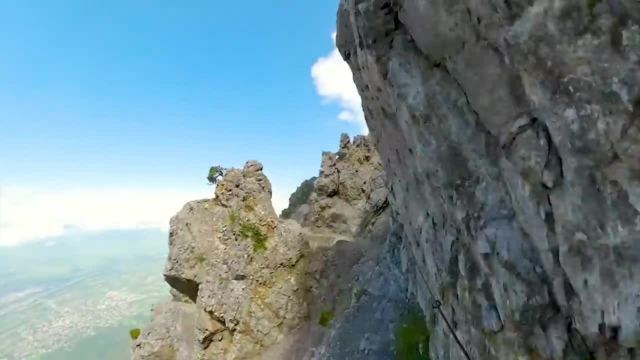 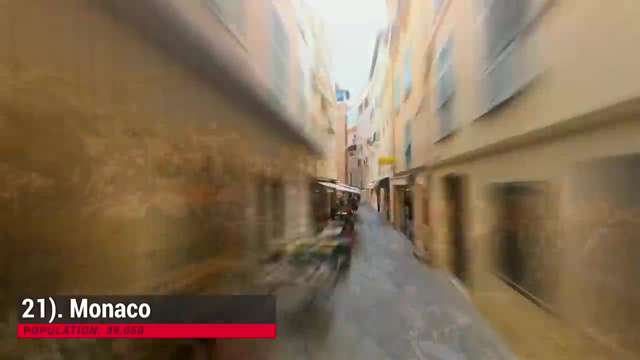 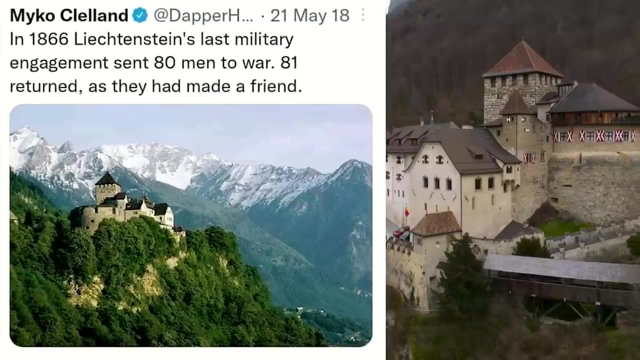 world's second-highest GDP per capita and third-highest life expectancy. Number 21, Monaco. Monaco's population is similar to Liechtenstein's, yet it's 80 times smaller, at a mere two square kilometers, making it the most densely populated nation. But while even Liechtenstein doesn't take itself seriously. Monaco is the most try-hard country. It houses the most millionaires and billionaires per capita, the highest GDP per capita and a human development index over one which shouldn't be possible. Why? Because there's no income tax, So wealthy people. over the world move here to flaunt their yachts and supercars. Number 20, Estonia. Estonia's capital, Tallinn, is less than a three-hour ferry ride from Finland's capital, Helsinki, And while it may seem amusing that countless Finnish tourists ride this ferry simply to buy cheap booze, it underscores. 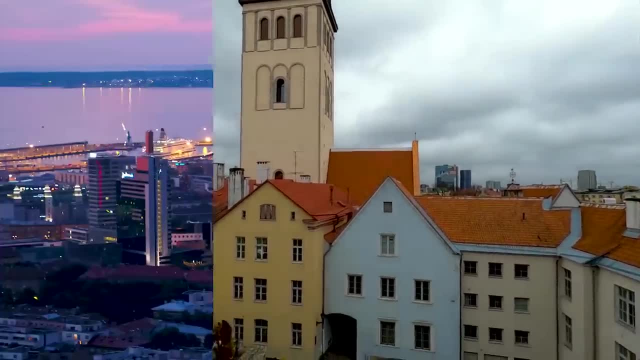 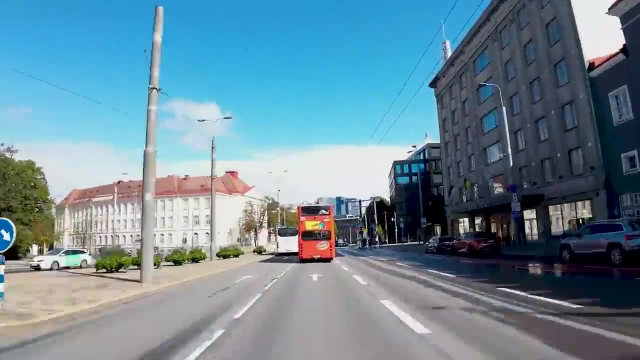 why Estonia is the most affluent Baltic nation: Trade and investment from Finland and Sweden. Estonia has also mimicked many of the Nordic nation's best traits, prioritizing education, safety and innovation, which is why it's the most affluent Baltic nation. 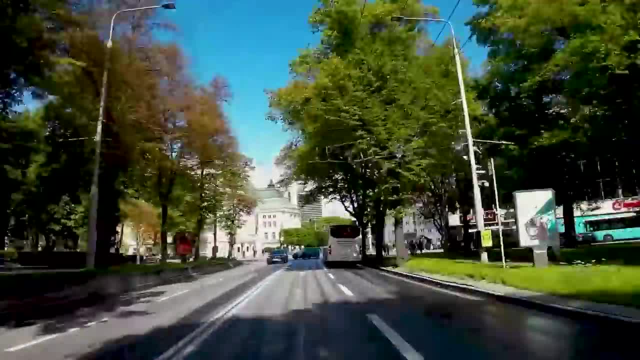 Estonia has also mimicked many of the Nordic nation's best traits: prioritizing education, safety and innovation, which is why it's the most affluent Baltic nation. Estonia has also mimicked many of the Nordic nation's best traits: prioritizing education, safety and innovation, which is why it's the most affluent Baltic nation. 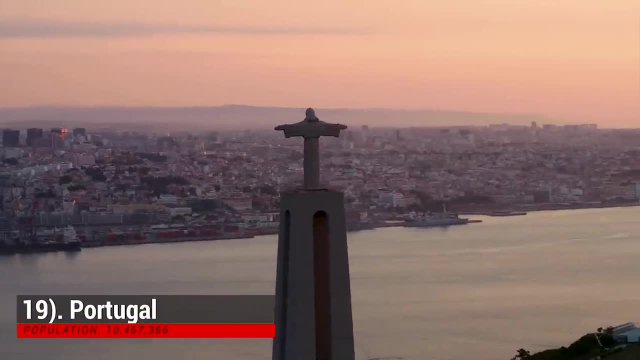 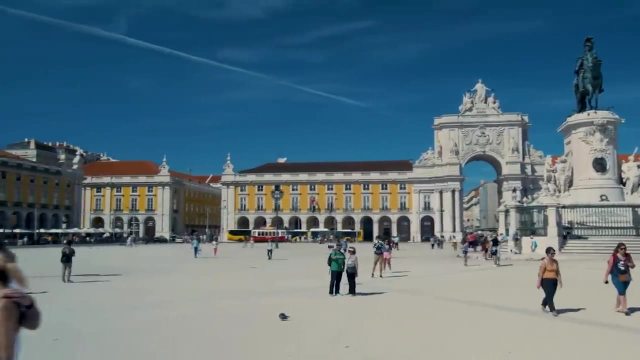 Number 19, Portugal. You may have heard of Portugal being a top expat destination due to it offering all the food, beaches, history and culture of most Western European destinations, while being a fraction of the cost, But since local wages aren't great, this has also created Europe's worst housing crisis, with home prices rising 157% from 2020 to 2021.. Number 18,: Cyprus. Cyprus has more billionaires per capita than any non-microstate nation, mainly due to its great weather and friendly tax structure incentivizing foreign tech companies to set up shop here. 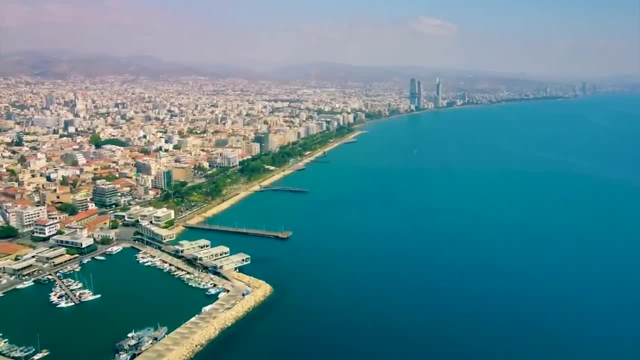 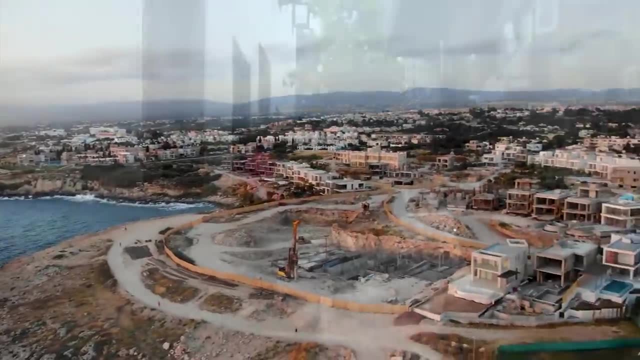 The island is a hub for forex, fintech, iGaming and crypto, not to mention the center of the online porn industry. But it's not just the wealthy who prosper. Average wages are similar to Western Europe and the healthcare is among the best in the world. 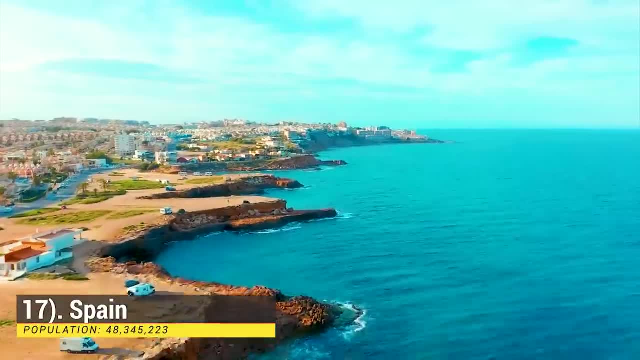 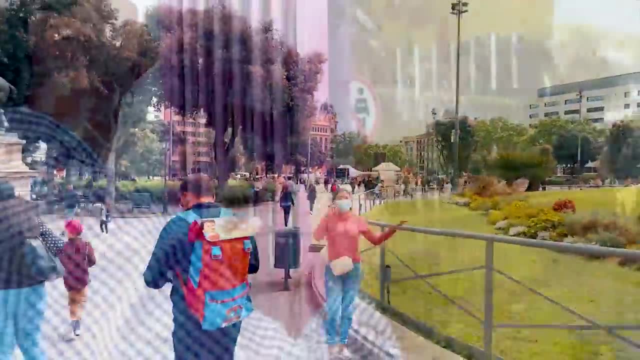 Number 17, Spain. Spain might have the best work-life balance of any nation. Not only are 30 paid vacation days and 14 paid public holidays required by law, many companies even close for 2-3 hours during the day for siesta. 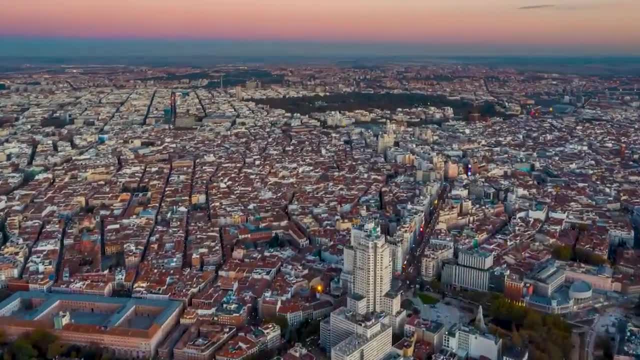 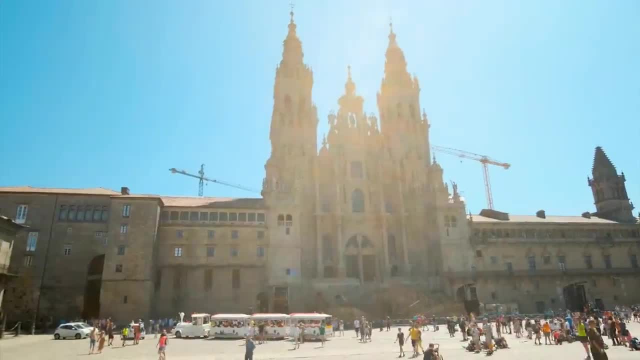 But while there's splendid weather, scenery, history and culture, in addition to some of the best food and drink on Earth, it's not all sunshine and wine. The 12.7 unemployment rate is the highest in the EU and the cities have Western European prices. 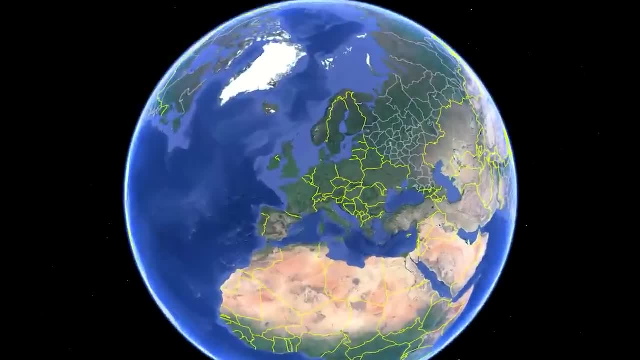 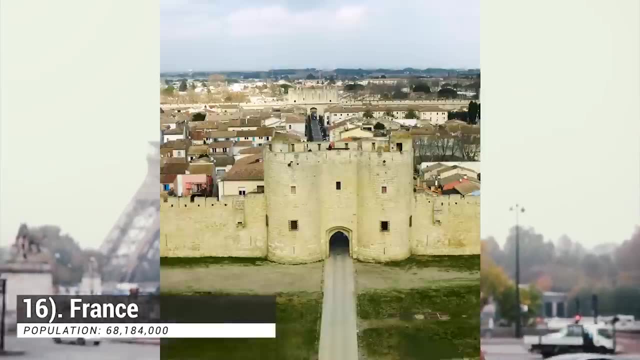 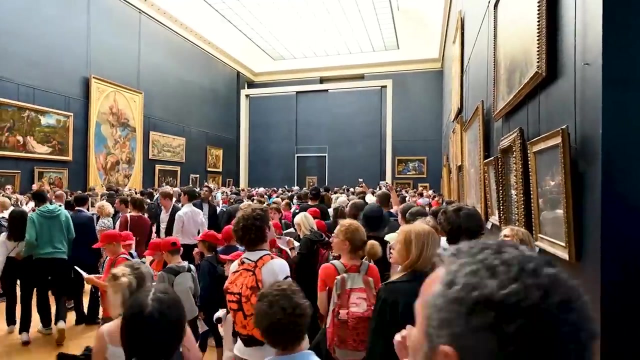 with Central European salaries, Number 16, France. When polled on who the most arrogant Europeans are, the French chose themselves because they have everything most people could ever dream of and they know it. The cuisine is out of this world. the arts and culture are unmatched. 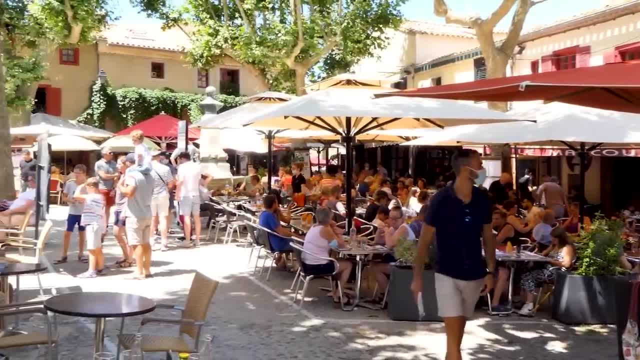 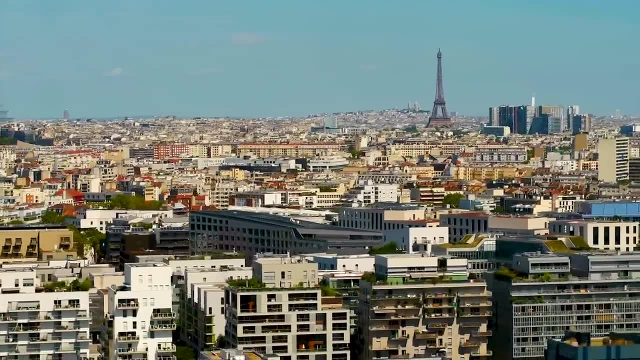 and the laid-back lifestyle emphasizes life over work. But that doesn't mean the French are lazy. They produce the world's 7th largest economy, and their healthcare, education and public transit are all outstanding. Number 15,: Czech Republic. Czechs are the. best in the world, and their healthcare, education and public transit are all outstanding. Number 15, Czech Republic. Czechs are the best in the world, and their healthcare, education and public transit are all outstanding. They produce the world's 7th largest economy, and their healthcare, education and public transit are all outstanding. 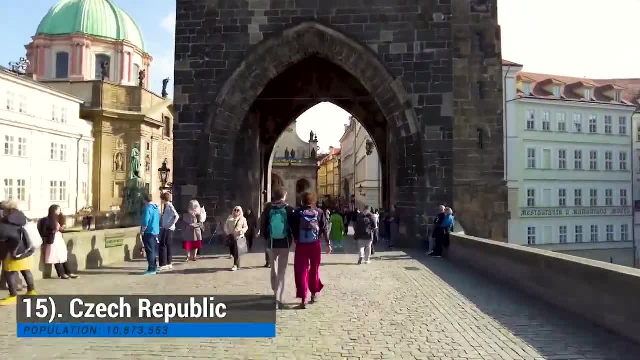 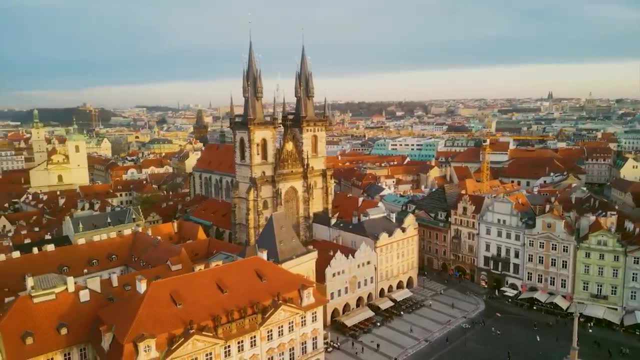 They produce the world's 7th largest economy, and their healthcare, education and public transit are all outstanding. Literally, the average Czech drinks 520 beers a year, which is nearly double the next country. But that's not the only thing Czechs excel at: The Czech Republic is home to the lowest unemployment. 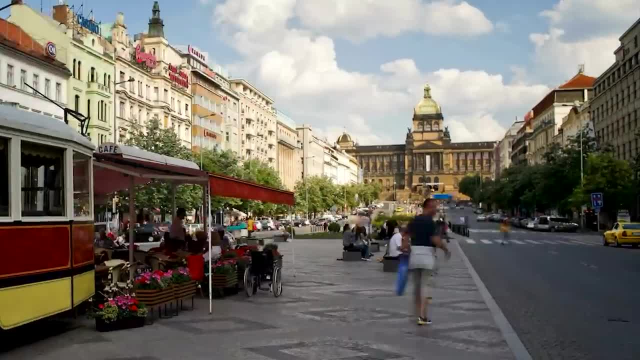 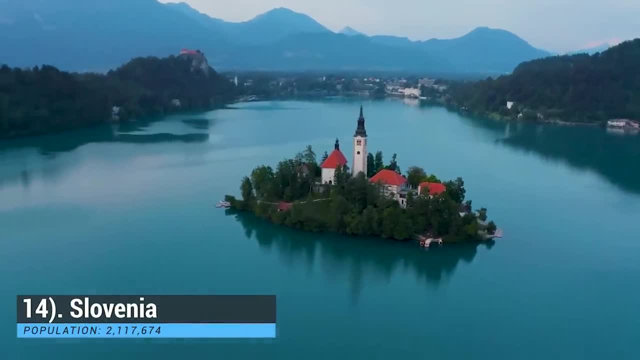 poverty and homicide rates in Europe, as well as one of the fastest-growing economies Number 14, Slovenia. If it weren't for Luka Doncic, most people would have no idea where or what Slovenia is, And that's a shame. 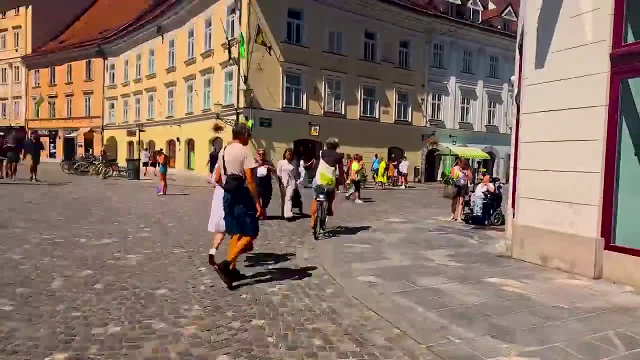 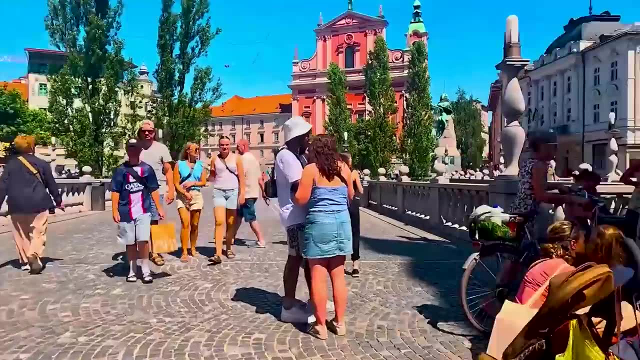 because, in contrast to most former Yugoslavic republics, Slovenia has had some of the best economic developments on the continent, with the GDP per capita tripling in the last 20 years. Plus, one in every 20 Slovenians is a beekeeper. because one: Slovenians love honey and two: 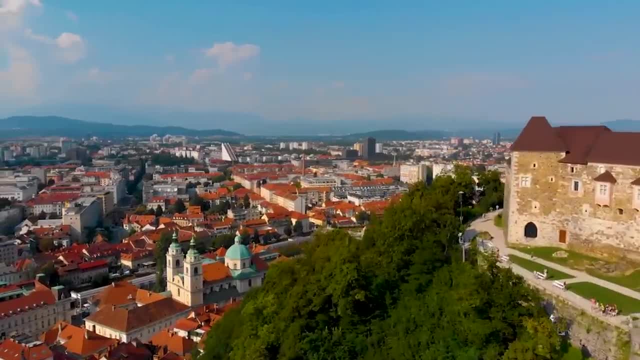 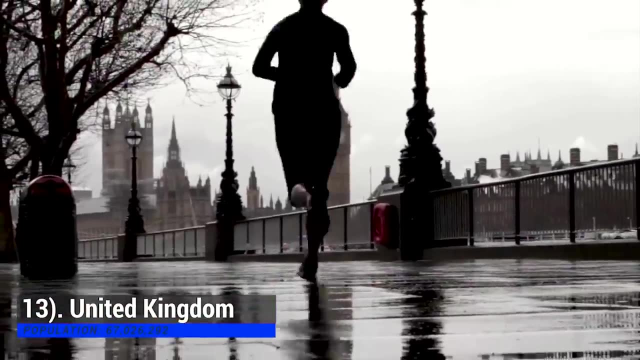 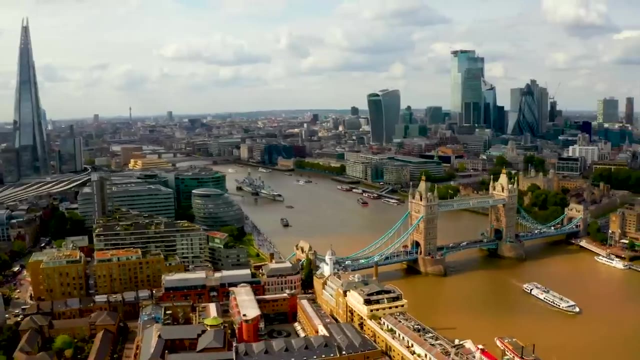 they prefer to shop local, which is a huge reason why Slovenia has the world's lowest income, inequality Number 13,. United Kingdom. The UK's damp, cold, gloomy weather is a metaphor for the nation's current sentiment Depressing. The average quality of life has steadily decreased since Brexit and 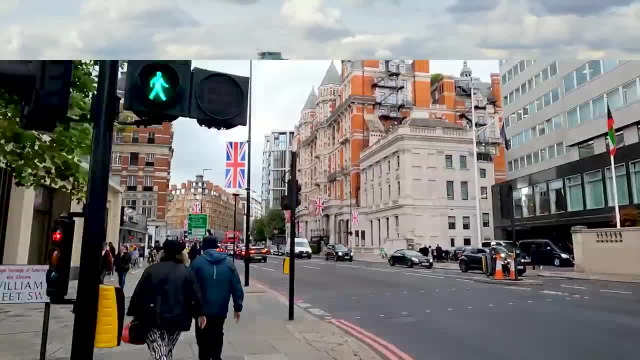 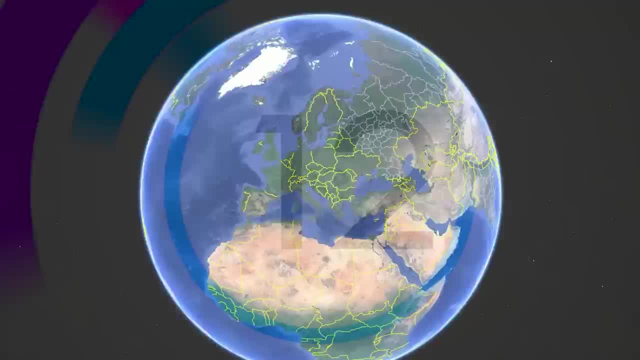 the economy has been in stagnation for far longer, But the UK is still the world's sixth-largest economy and the free public healthcare and education is excellent. Number 12, Luxembourg. Sure, it's boring, but stats don't lie. 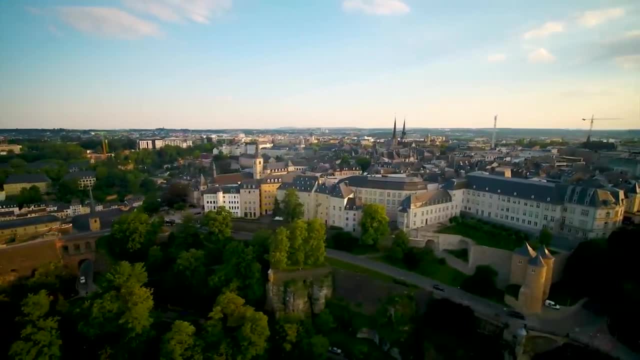 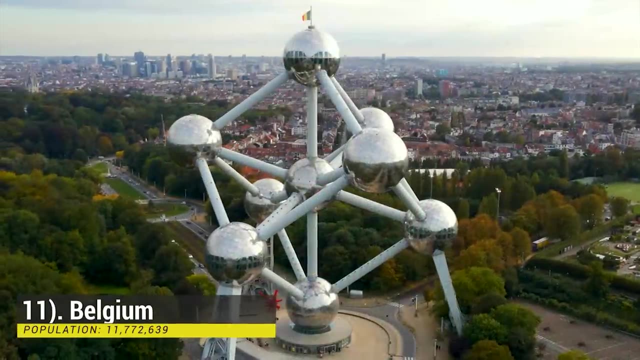 and neither is the highest GDP per capita on Earth. But Luxembourg is also outrageously expensive. Number 11,, Belgium, Home to the EU's capital and bordered by the Netherlands, Luxembourg, Germany and France, Belgium is a mix of the best-growing countries in the world- The best-growing 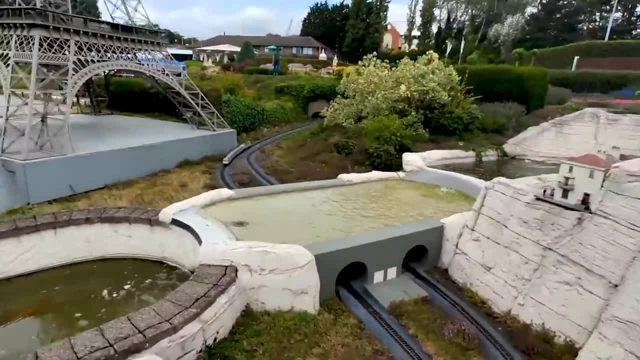 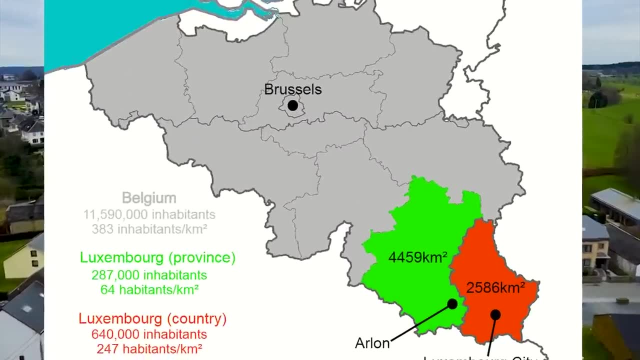 parts of those nations crunched into a smaller, more urbanized version. Well, maybe not exactly smaller, because Belgium has a province called Luxembourg and that alone is 71% larger than Luxembourg. But similar to Luxembourg, Belgians are incredibly wealthy. Nearly three-fourths of the population owns their own home and the median wealth per adult is the third-highest in the world. Number 10,: Austria. From schools to healthcare, the economy to safety and everything in between, Austria is among the top 15 nations in literally every category, including the most paid time off. 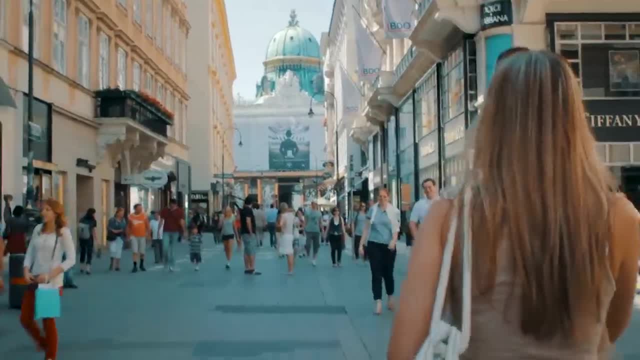 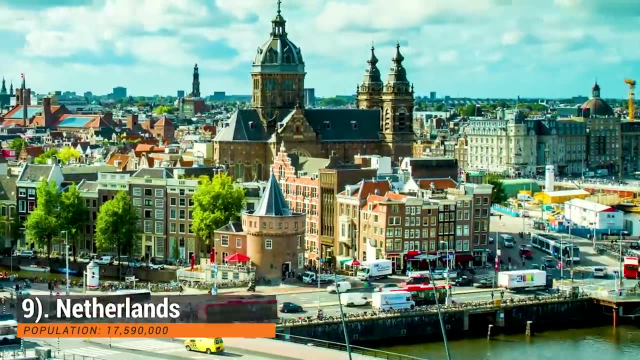 Plus, it's jaw-droppingly beautiful and Vienna is often ranked as the best city on Earth. Number 9,: The Netherlands. While many argue that Monaco, the Vatican and other microstates shouldn't exist, the Netherlands literally shouldn't exist: 26%. 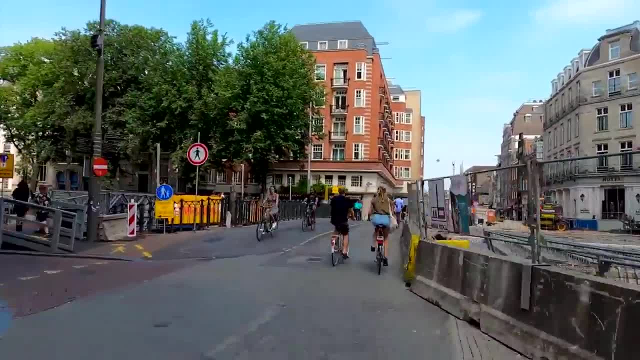 of its area is located below sea level, But the Dutch's ingenuity and resourcefulness of building dykes, pumps and canals, which allow 50% of the country to live in the Netherlands- and the Dutch also have a lot of money to spend on the economy- are not enough to make the country a better place to live. 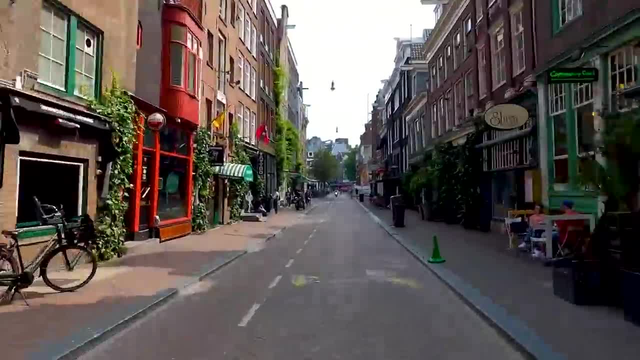 But the Dutch's ingenuity and resourcefulness of building dykes, pumps and canals which allow 50% of the country to live in the Netherlands. pumps and canals which allow 50% of the country to live in the Netherlands. 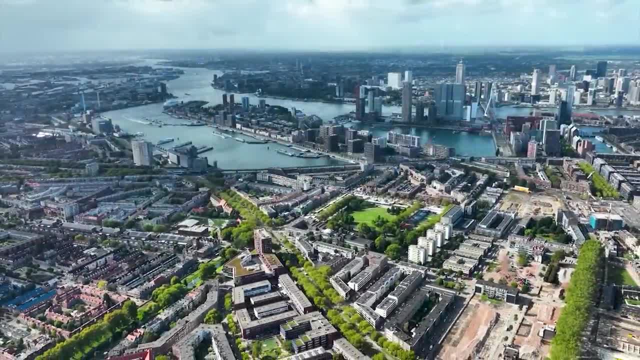 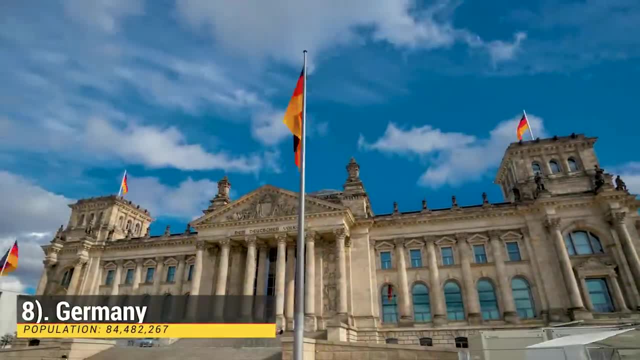 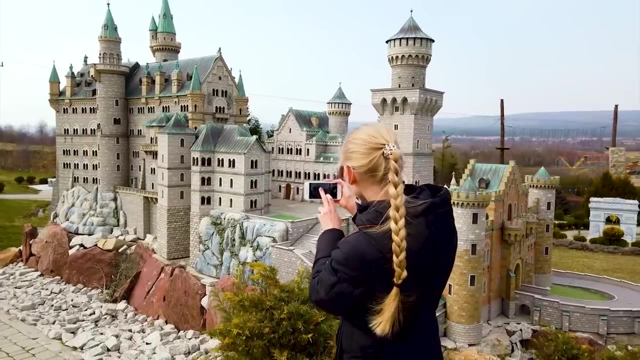 has also translated to its economy, with the Netherlands having the third highest after-tax net income of any nation. Number 8, Germany. Germany is the economic powerhouse of Europe, having just surpassed Japan to become the third largest economy. all while Germans work less hours than any other nation. How Well they're highly educated. 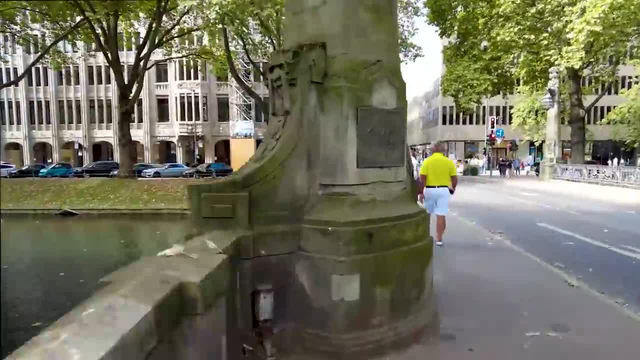 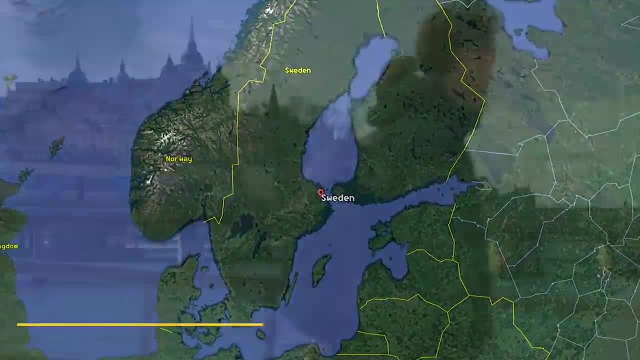 and because they don't work as much, Germans are much more productive in the time they do work, since they know they'll have plenty of time to socialize and enjoy life after Number 7, Sweden. Sweden is perhaps the perfect balance between capitalism and socialism. 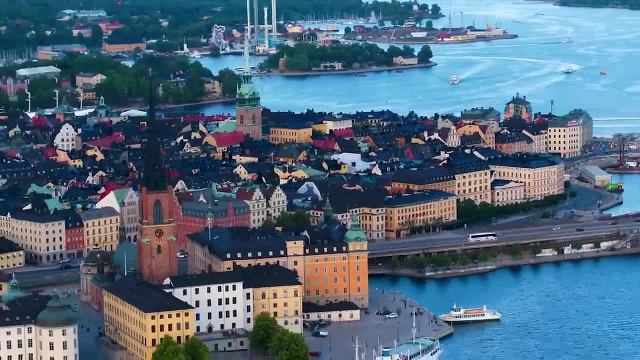 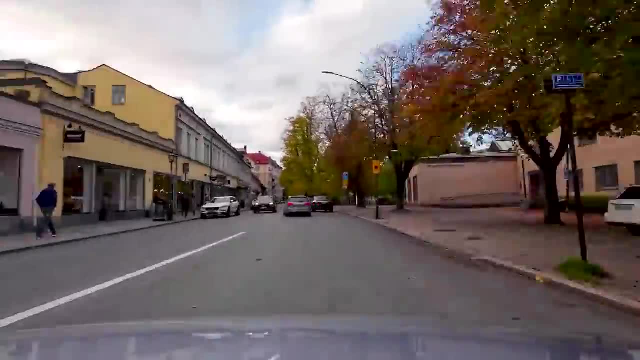 with the Scandinavian nation being home to one of the best economies, due to low corporate taxes and plenty of innovative companies, while also having an incredibly strong social safety net. Heck, the government even allows Swedes to take 6 months off in order to start their own business. 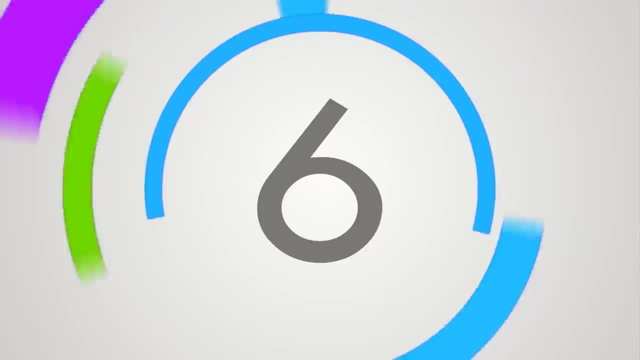 with a guarantee they can return to their job if their idea flops. Number 6, Sweden. Sweden is the only country in the world that has a high social security net. Sweden is the only country in the world that has a high social security net. 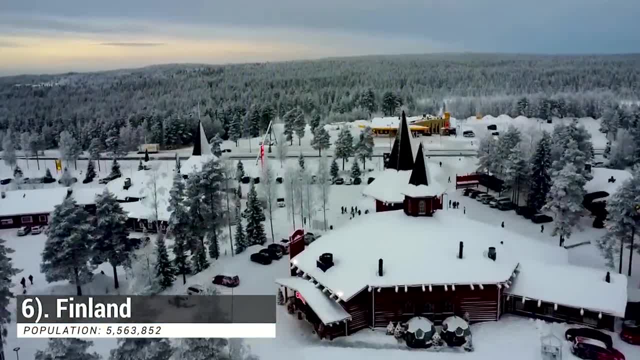 Sweden is the only country in the world that has a high social security net. Finland. Less than 6 hours of daylight and brutally cold winters might seem depressing, but Finland has actually been the happiest nation for 8 years running, which goes to show how much 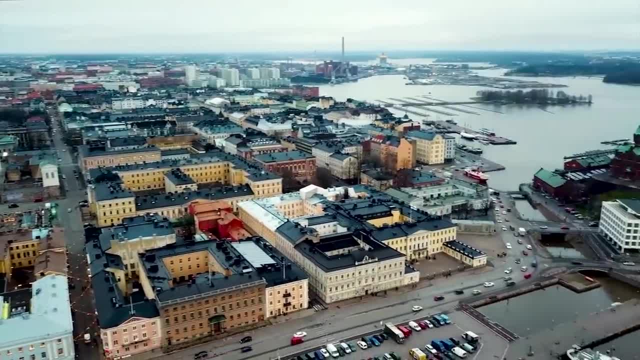 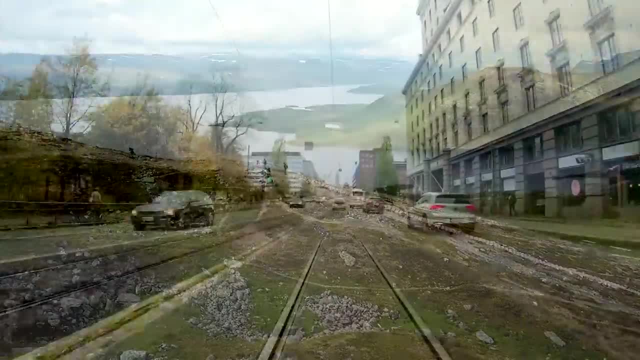 a non-corrupt government that cares about its residents can increase a nation's quality of life, Because, with the world's best schooling system and parental leave policy, the cleanest air and water quality and highest level of food security, Finns have little to stress about. 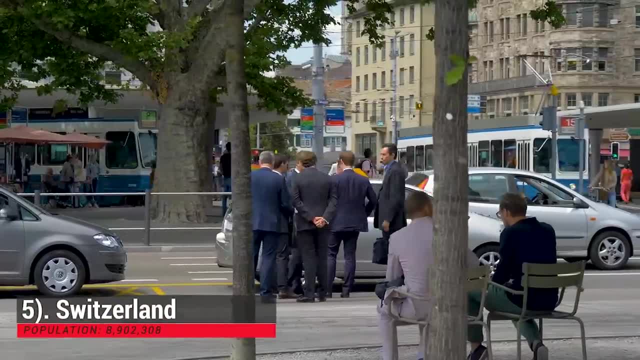 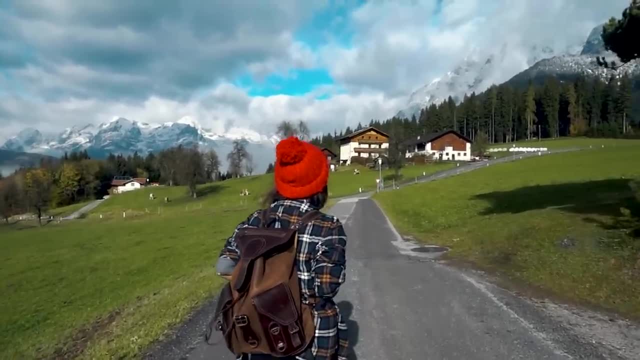 Number 5, Switzerland. Nothing in life is free, and there's a reason: Switzerland is ridiculously safe, with the world's best public transportation, healthcare and after-tax net income, Because it's also the most expensive nation. But boy, is it beautiful. 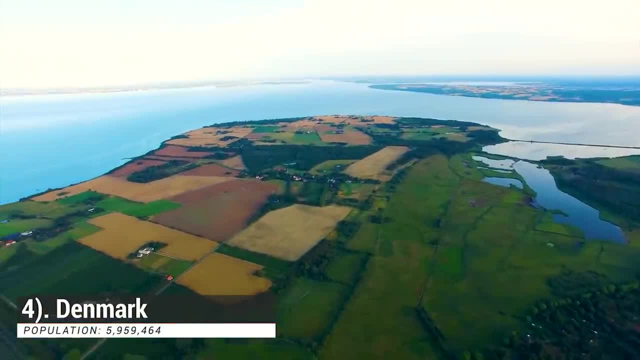 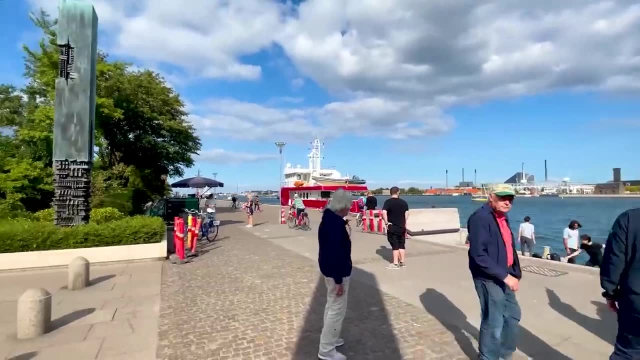 Number 4, Denmark. Denmark may not have the best museums, food or natural scenery, but when it comes to the essentials, such as good paying jobs, cleanliness, safety and great quality affordable healthcare, education and housing, few nations do it better. than the Danes. Number 3, Ireland. Ireland has the highest PPP GDP per capita, at $145,000,. a full 65% higher than Switzerland, the second wealthiest non-microstate, But despite its already exceptional economy, it's also the fastest growing, with a 9.4% annual GDP growth rate. 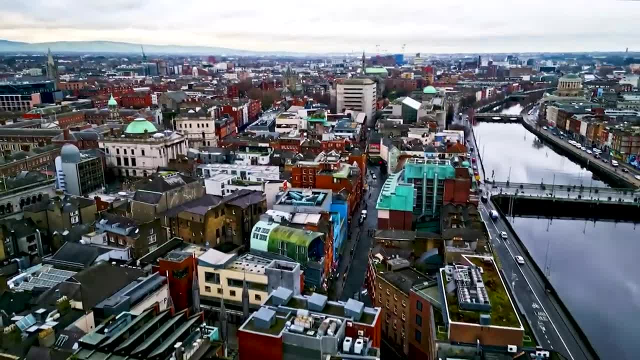 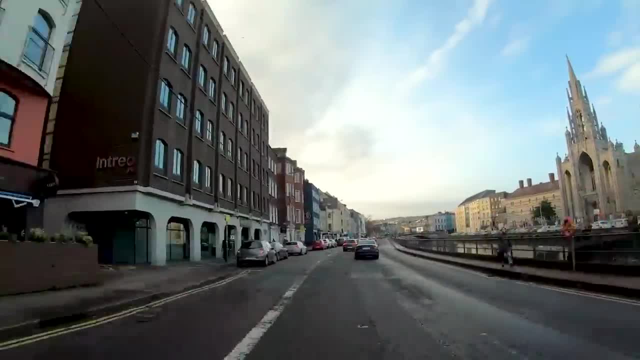 How do the Irish keep finding massive pots of gold? Well, it's home to Europe's most educated working class and corporate-friendly tax laws, resulting in nearly every large US company placing their EU headquarter in the UK. The UK is the largest country in the world, with a population. 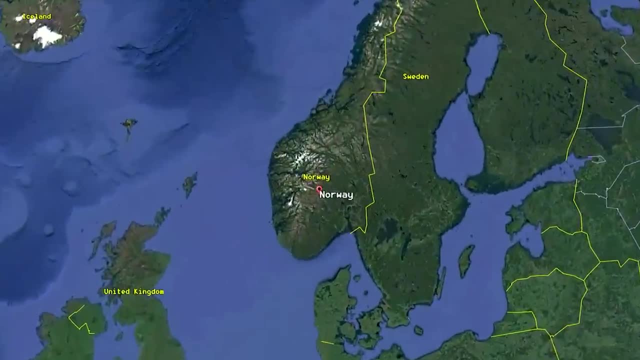 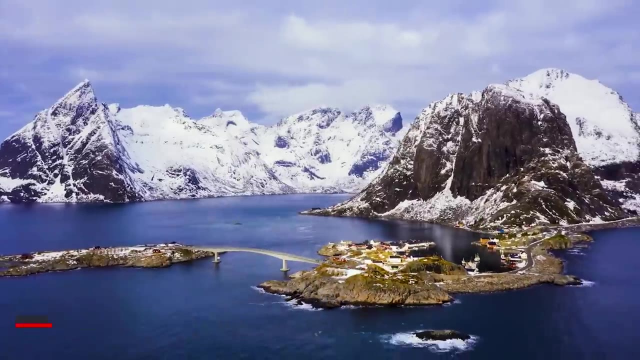 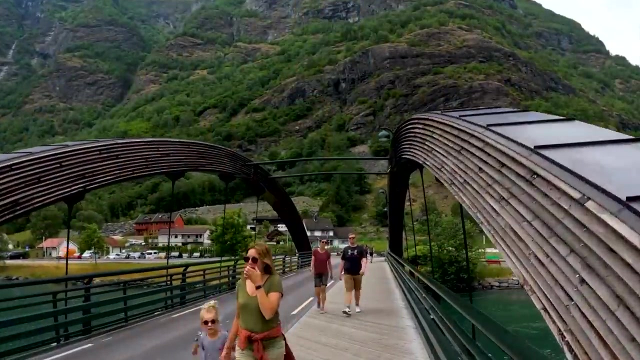 of 1.4 billion. Number 2, Norway. Norway is a hypocrite. It's one of the cleanest, greenest nations, with 97% of its trash being recycled, 99% of its energy coming from renewable sources and more electric cars per capita than any other nation. Yet a big reason why it has 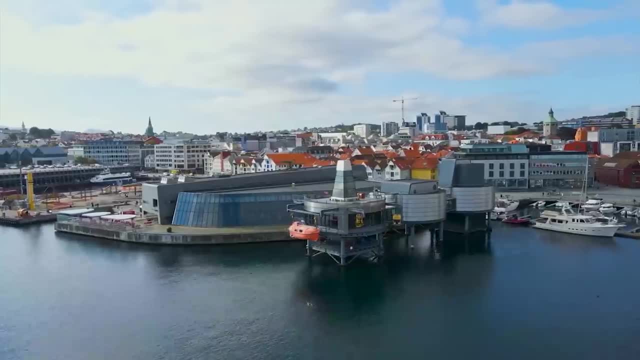 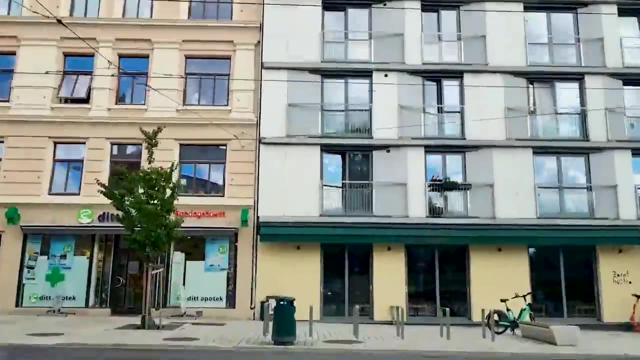 the world's third highest nominal GDP per capita is due to it being one of the biggest exporters of oil. This also pays for Norway's superb social programs, however, with 59 weeks paid family leave, a top-five healthcare and education system and a highly successful qualification program. 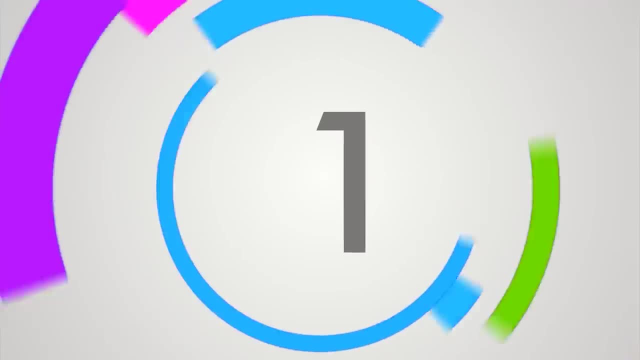 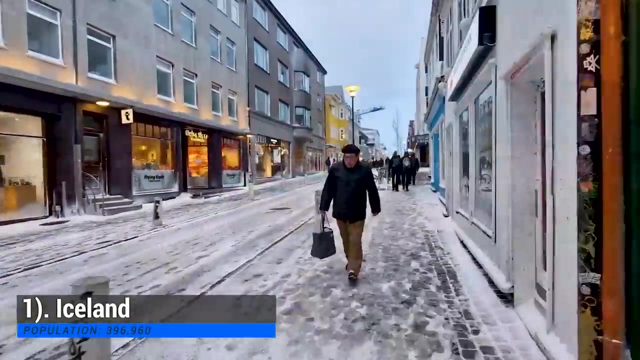 which pays unemployed people to learn new skills. Number 1, Iceland. Iceland is the epitome of how incredible a non-corrupt nation can function, Having been democratically run for over a thousand years. every penny the government takes goes back to helping its residents.